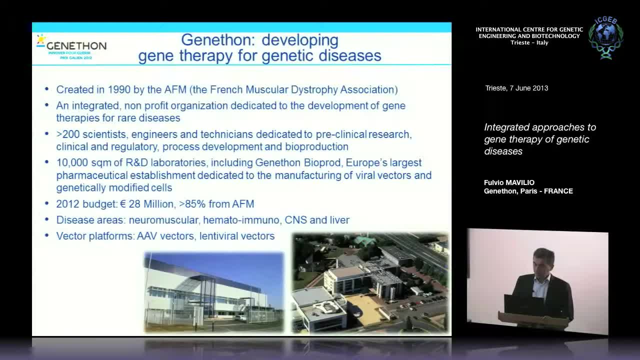 the same thing. It's a charity and it's focused on rare diseases. It was originally created in 1990 by the AFM. The AFM is now it's called AFM Teledon, but it's essentially it was the French Muscular Dystrophy Association, which now focuses in general on rare genetic. 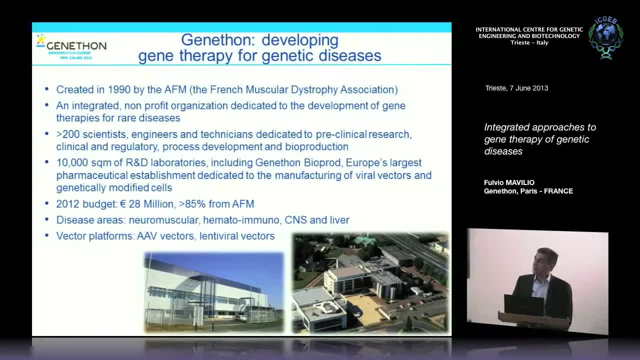 diseases. At the beginning, Genedon started as part of the Human Genome Project and it actually had the very significant impact on the human genome And it was a very significant role there, because it was in Genedon that the first haplotype map of the human genome. 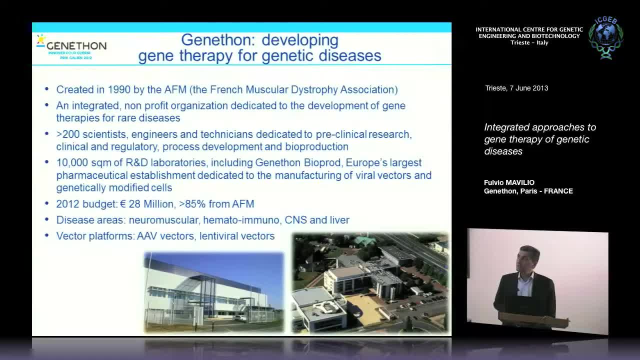 was finished and published in Nature in 1990 or 91, something like that- And eventually in 95,, under the direction of Olivier Danos, became an Institute of Gene Therapy. So it's a big thing, as you can see here. This is the research. 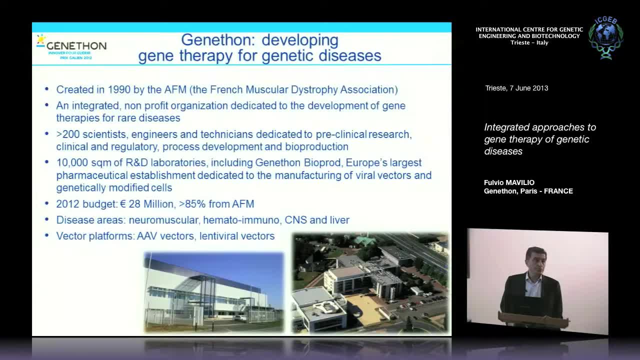 This is the research building and plus, this is the virus production building. I will give you a hint during my presentation of what is this building for And, as I said, it's completely funded- almost completely funded- by the Teledon and it's a non-profit organization. 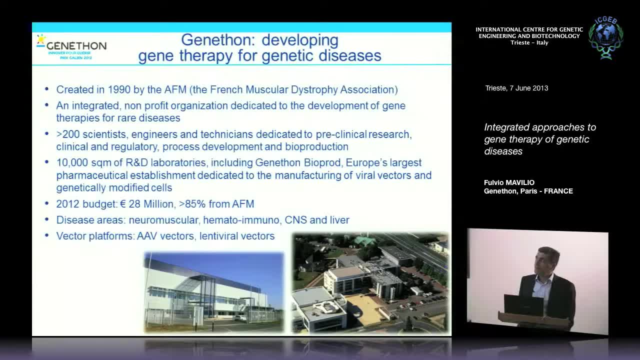 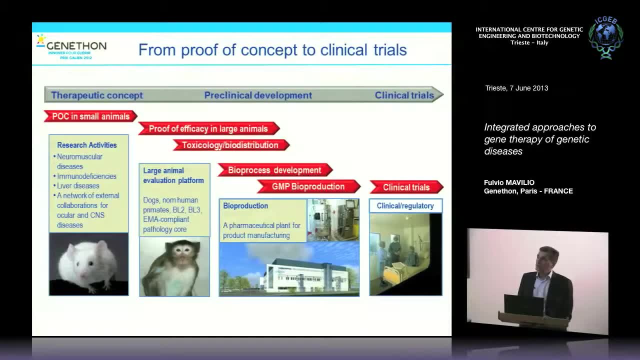 dedicated to gene therapy of neuromuscular blood, CNS and liver diseases. Genedon is a completely integrated organization. So we do preclinical research, we do experiments in the laboratory. of course We have animal platform for small animals, large animals. 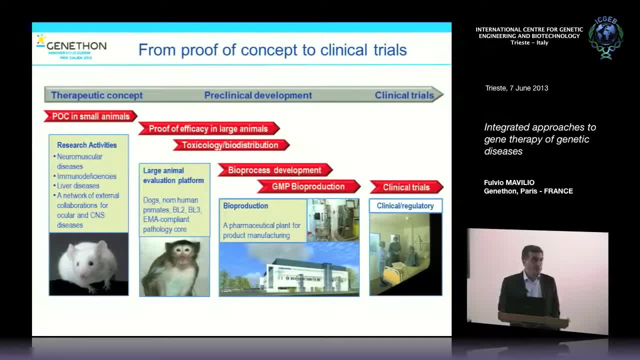 a full GMP pharmaceutical establishment that can produce in GMP both lentiviral vectors and AAV of different serotypes, And we have a network of collaborations, many of whom I'm sure you know very well, for the clinical application of the virus And the research. 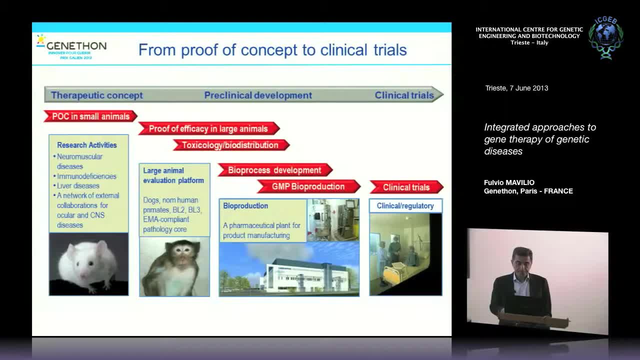 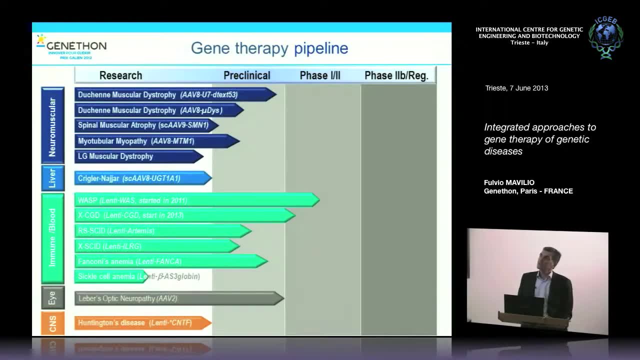 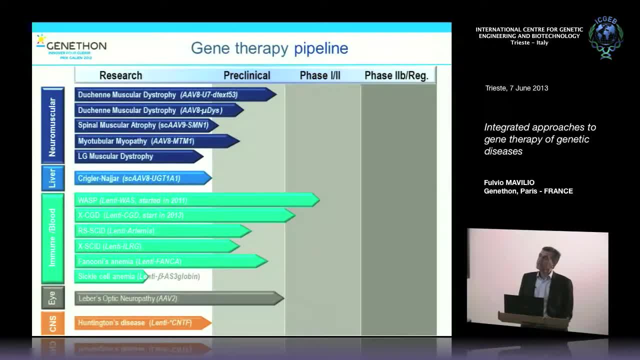 we are working on And if you look at this pipeline, you can essentially say that this is completely crazy- which is what I said the first time I stepped in- And it's essentially a big program on neuromuscular diseases. not surprisingly, This is the mission originally. 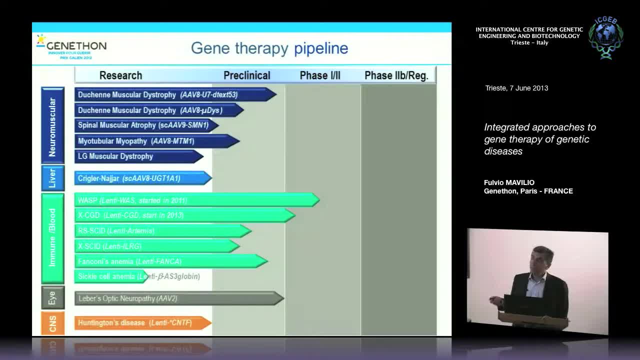 of Genedon, Something on the liver, a big program on blood genetic diseases and then on the liver. So this is a big program on the liver, a big program on the liver, a big program on blood genetic diseases And let's say, other programs on the eye and CNS diseases which 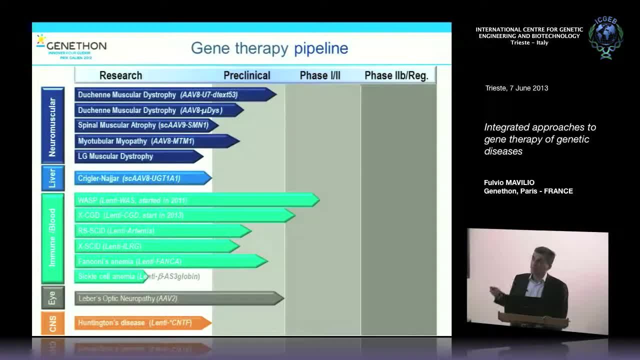 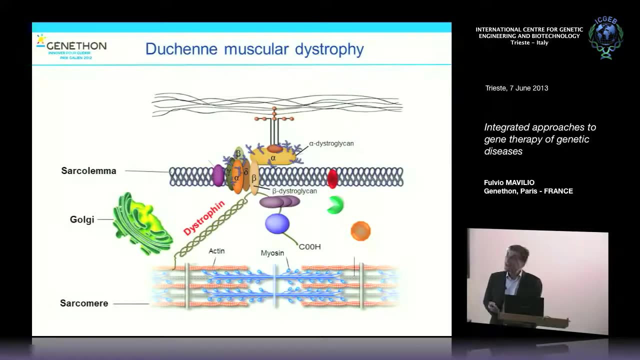 are essentially done in collaborations, But most of the effort and everything I will show you today is focused on the neuromuscular program and the blood genetic diseases program. I will start by so. what I will do is essentially give you an idea of what we are doing in these. 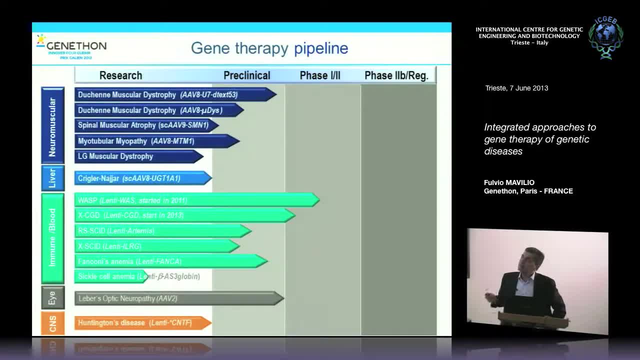 two fields And I selected a few stories that give you an idea of the type of approach and how likely it is that some of these therapies will reach the clinical phase soon or very soon, or they are already there. I will make a couple of examples in the field of muscular dystrophy and, in particular, Duchenne. 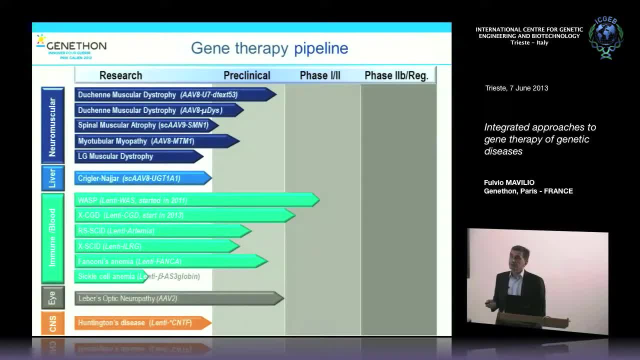 and myotubular myopathy And I will give you some examples in the field of neuromuscular dystrophy And I will give you some examples in the field of blood disorders and, in particular, for some immunodeficiencies. So these are examples of in vivo gene therapy based on AAV, essentially, and ex vivo based. 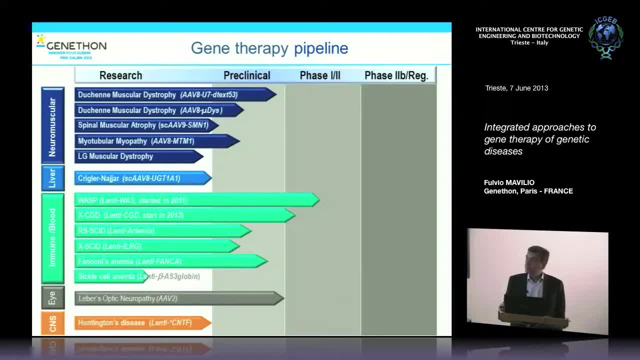 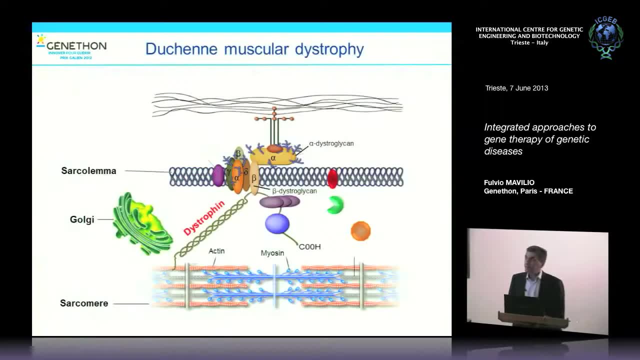 on stem cells transduced by lentiviral vectors, So genetically corrected stem cells transplanted into patients. So let me start from the Duchenne muscular dystrophy. As many of you- probably most of you- know already, this is the most frequent genetic muscular dystrophy in men And it's 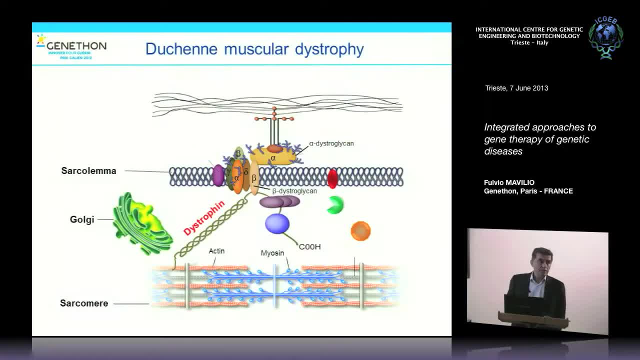 due to deficiency of this huge protein- It's called dystrophin- or dystrophin, depending on what side of the Atlantic Ocean you live- And which is a big filamentous protein that is essentially a bridge between the contractile machinery of the muscle fibers and the extracellular. 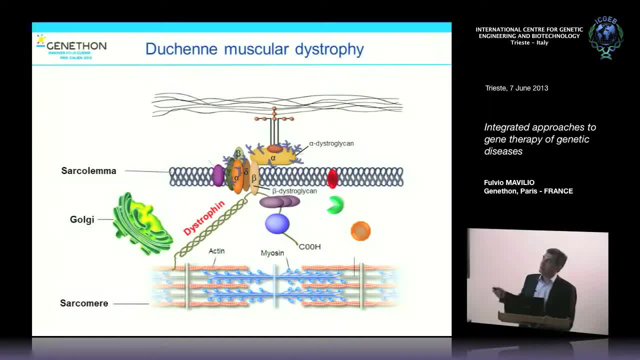 body extra fiber environment. so this multi-molecular bridge which goes through the sarcolemma membrane is important and it's important it is intact. if there are there is deficiency in any of this sarco-glycan or distro-glycan or dystrophin proteins, the this connection is disrupted. 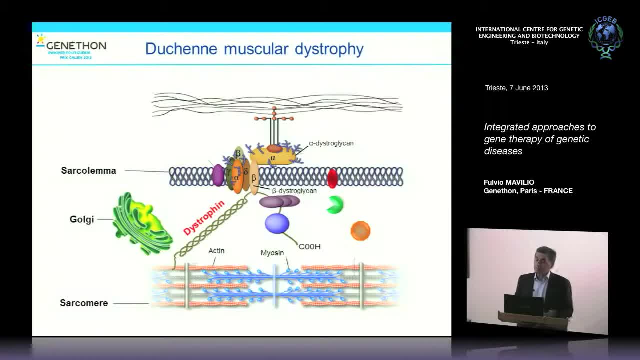 the muscle fibers degenerates and create and gives rise to what we know as muscular dystrophies, which is a family. the Duchenne is due to deficiency of these proteins. there are many mutations, deletions, point mutations. it's a collection of those, but essentially the problem. 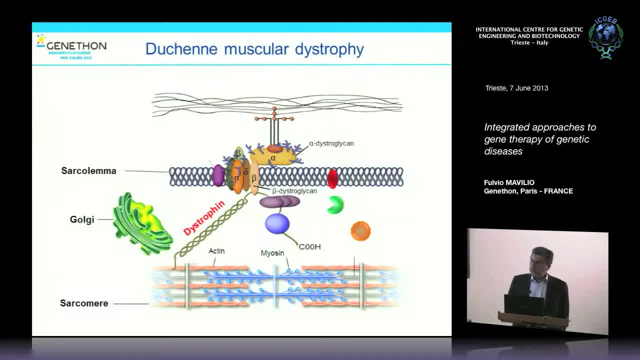 is that you don't have enough of this protein. so theoretically an easy problem. you go, you restore this protein synthesis and you cure the disease theoretically. theoretically, practically, is extremely difficult for a number of reasons. the first is that the dystrophic phenotype, once it is established, is not reversible once you have lost your muscle. 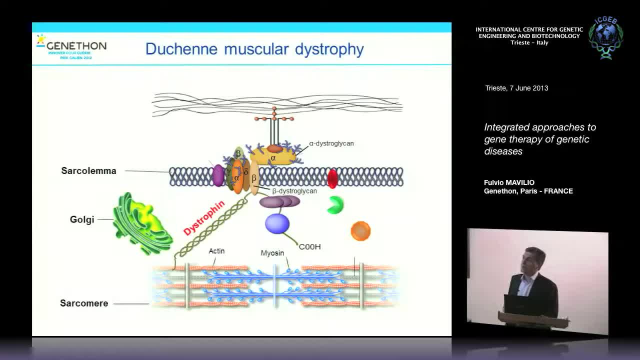 function, that is, and your muscle tissue is replaced by by scar tissue, essentially by fibrotic tissues. there's no way you're going back. so the only way is to prevent the degeneration, which means you have to go into children, you have to go into early phases of the 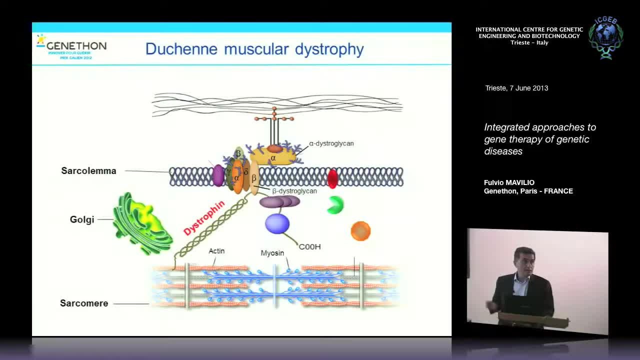 disease. the second is that this protein is huge. this, the DNA, the cDNA that can code for it, not to mention the gene that is 2.5 megabases, is very difficult to to transfer. and and the third, that it's the- the muscle is most of our body mass, so you have to reach in vivo an enormous amount of 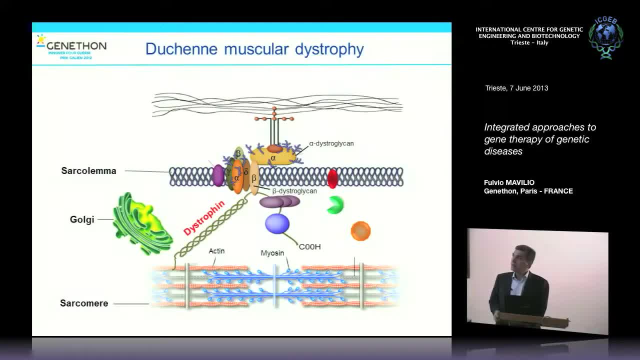 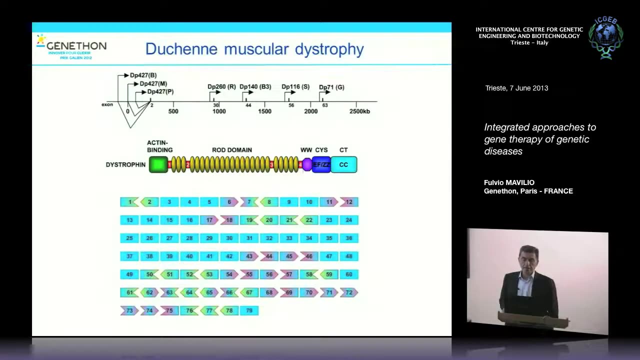 target tissue. you can now just target a stem cell. so all together this makes the most formidable challenge for a gene therapy approach and, not surprisingly, very little as worth up to date, except for the mouse model, which is relatively easy to correct. So many years ago, at genet on, Luis Garcia and Olivia Danos started working on a potential 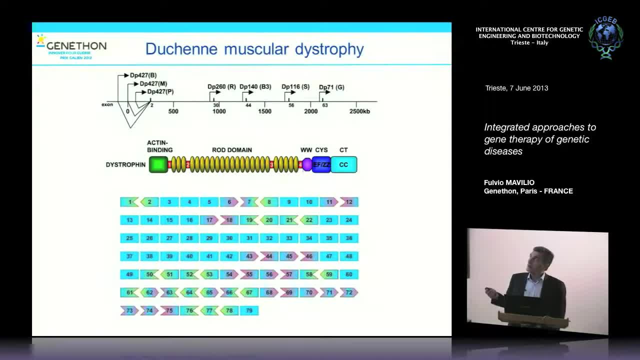 approach which is called excellent keeping. so, as I said, this is the district and produce of an N-terminal domain, a carboxy-terminal domain and a very long road domain, which is a repeated thing, And there are several mutations in several exons. 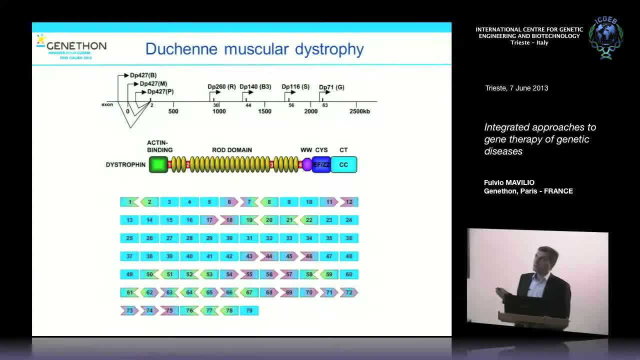 but essentially, when you have a mutation, one easy way to solve the problem without impairing the function of the protein is to skip the exon or the exons that are mutated and essentially restore protein synthesis by skipping the mutation. This is theoretically feasible in particular, for instance, 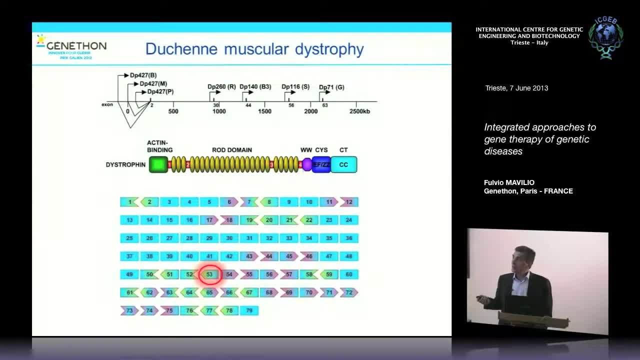 if you have a mutation in exon 53, which accounts for 8% of the mutation in patients, you may think of skipping these exons and bridging exons upstream and downstream and restore the frame and the protein synthesis. Now the shape of these little pieces here. 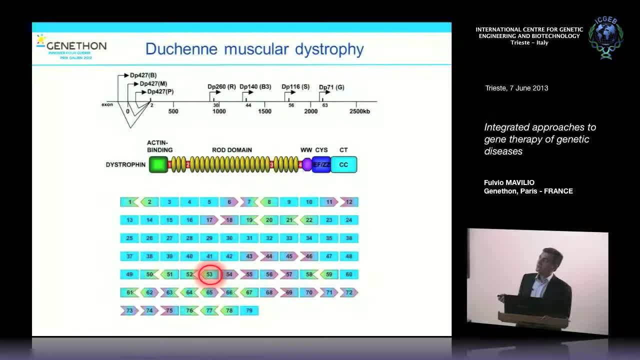 each one of these is an exon- gives you the idea that you have to put, of course, everything back in frame. So 43 is in frame with 44, but not with 45. So there is a code here that you have to respect. 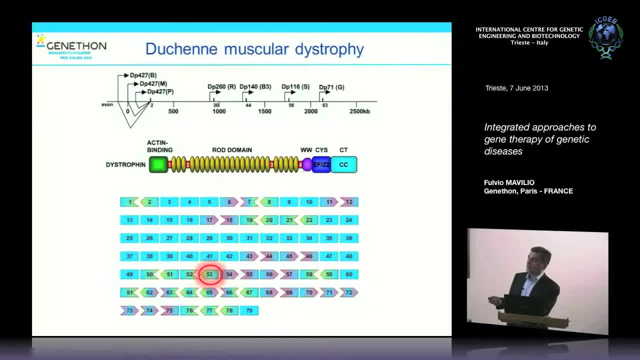 in order to do something meaningful. So if you want to skip 53, the easiest way is to go from 51 to 54. And if you have ways of skipping, of inducing exon skipping in the primary transcript of the gene, this is theoretically feasible. 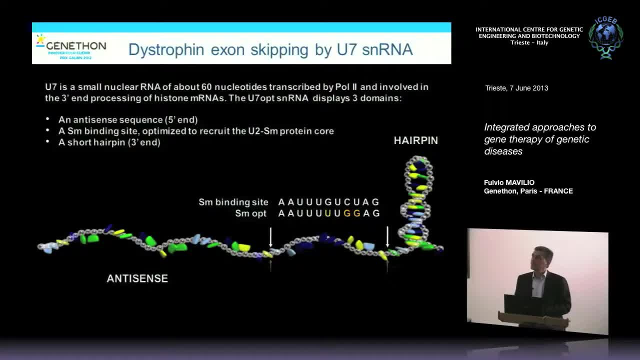 And what Luis and Olivier invented in essentially in the mid 2000, was to use, as a way to induce skipping, a small nuclear RNA that's called U7.. I have absolutely no time to tell you everything about this little RNA and what is its role. 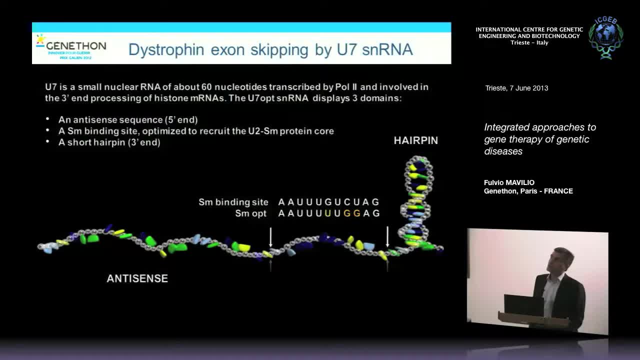 It's essentially part of the splicing machinery of histone mRNA, but it doesn't matter. It's essentially an RNA that has a binding site for a same protein, So it is targeted to the spliceosome And, if you can, if you build into this RNA and antisense part. 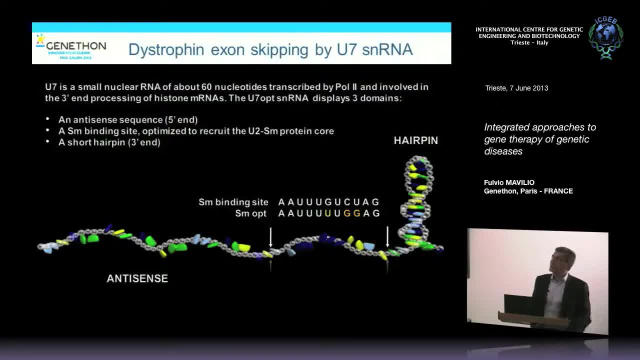 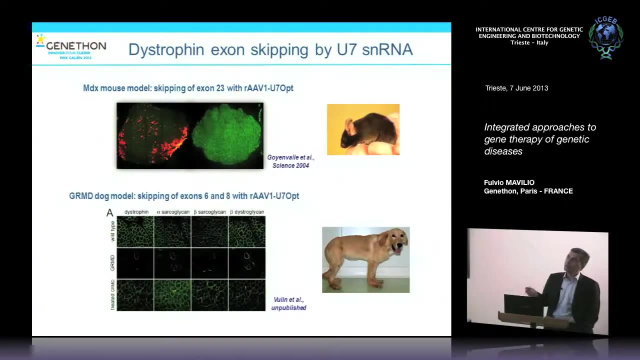 that it's a complimentary to part of what you want to skip. you essentially interfere with splicing and you can cause jumping and exon skipping. The proof of principle for this was given in 2004, in this seminal paper in science, in which they showed that 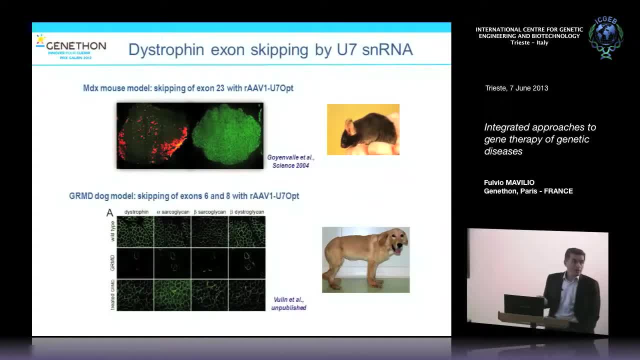 delivering this to a muscle. in the mouse model of muscular dystrophies, the MDX mouse skipping, exon 23, in this case in the mouse, was feasible And this restored protein synthesis in most of the mouse culture. So it was really very interesting paper. 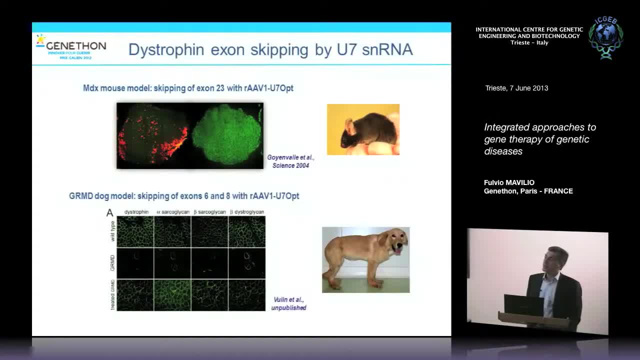 More recently, the group of Philippe Moullier, together with other people at Geniton, transferred this type of technology into the DOC model, which is much more difficult to correct. On the other hand, the DOC model is very much more similar to the human pathology than the MDX mouse is. 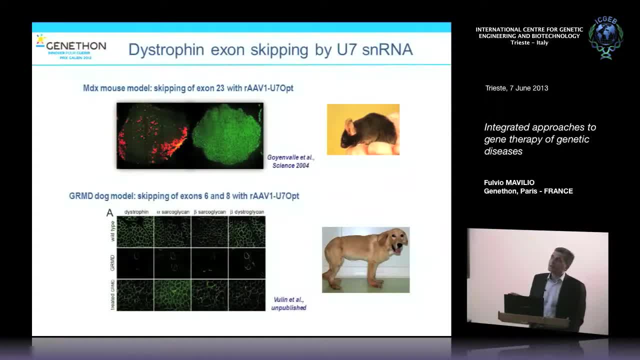 essentially showing by intramuscular injection, essentially the same thing. So you can restore the dystrophy synthesis, which is this green ring, into a GRM and DDOGS is a golden retriever- muscular dystrophy is called- and restore a protein synthesis. 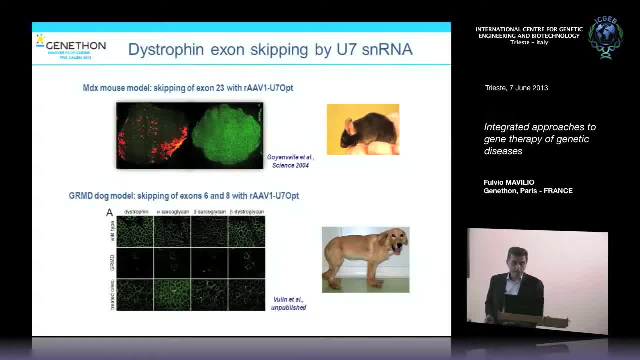 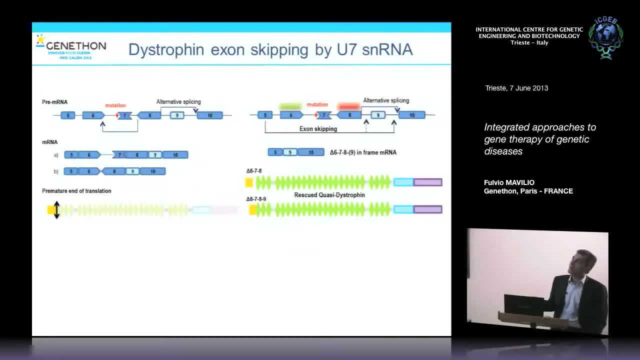 by skipping, in this case, exon six, exon eight. So how does it work in the DRM, in the dog? This is the model I would show you rapidly. There is a mutation. This is a natural model In the dog. it's a natural mutation And the mutation is here and essentially. 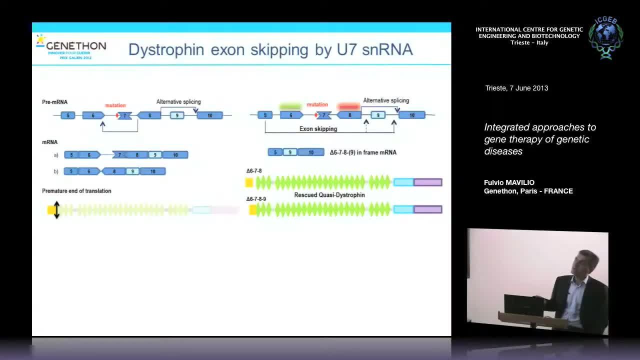 creates, interferes with splicing and essentially creates two RNAs, this one and this one, which cause premature end of translation. So essentially there's no protein synthesis. There is some exon skipping, naturally occurring, and residual protein synthesis, so that the dog is not completely 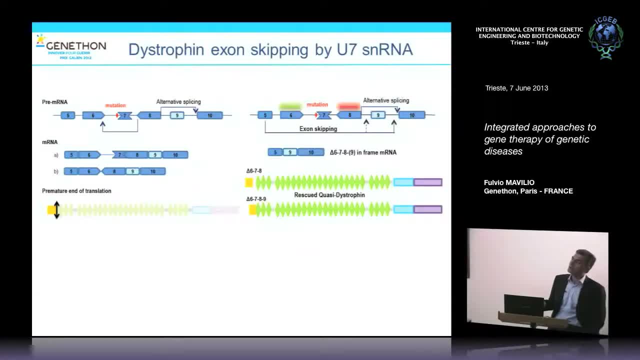 naive for the protein, But essentially it is a phenotype, So it's a dystrophic phenotype. What we can do we can do is using U7 to couple exon 6 and exon 8 to essentially introduce a skipping and go from and create a skipping between 9 and 10.. 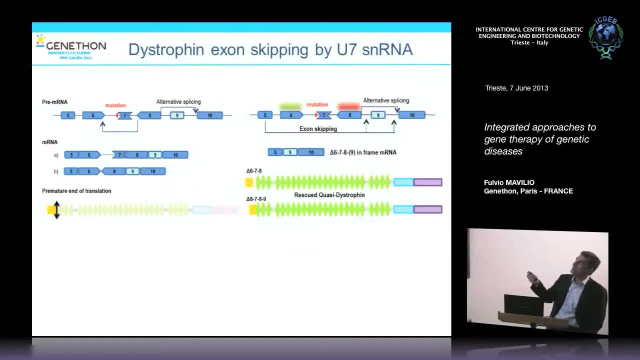 I'm sorry, 5 and either 9 or 10.. This is an alternative, splicing, of course, naturally, And obtain these two types of RNAs: delta 6,, 7,, 8, or delta 6, 7,, 8,, 9,, which are both. 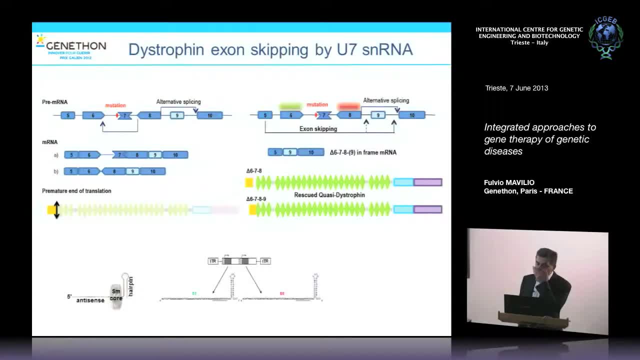 in frame and both code for the protein. So this is doable. It can be done by creating U7 RNAs modeled to these exons. These are here, And these two RNAs are both transcribed within an AAV vector, So they're both in the same vector. Of course, these are very 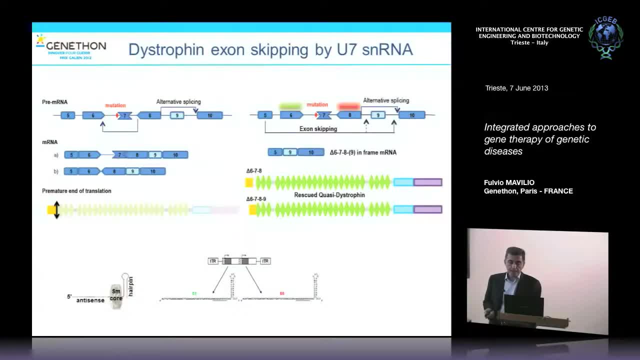 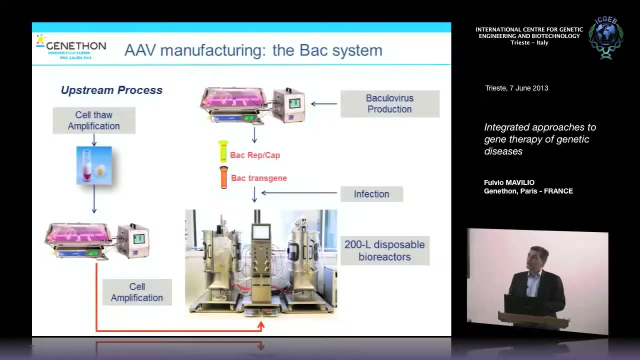 small genes and this can be packaged into a serotype 8,, for instance, which is very good for muscle like other serotypes, and injected into the dogs. I make a parenthesis just to: I know that some of you are involved in AAV biology, for 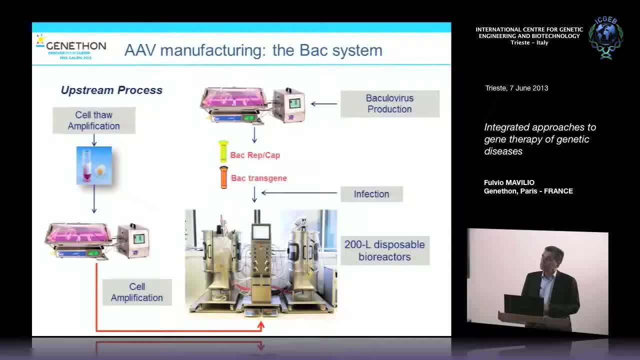 sure, and maybe also Virus. Yeah sure, synthesis and production and of course, this is a very crucial aspects when you want to go into a large animal model and, of course, in patients. so you have to produce very significant doses and what was developed during the years? a genadon. 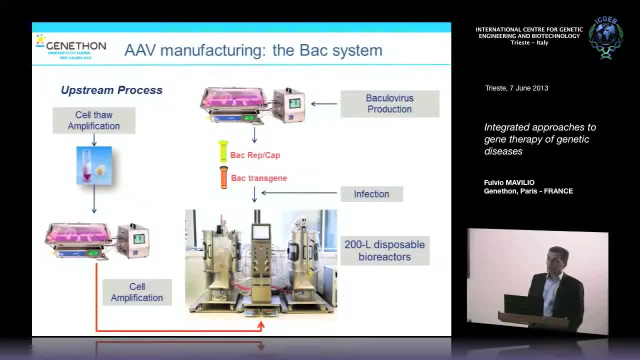 is a system based on baculoviruses, which, again, I don't have the time to to describe you in the details, but essentially is a virus that produces another virus. so it's based on two baculoviruses: one that calls for rep and cap, and 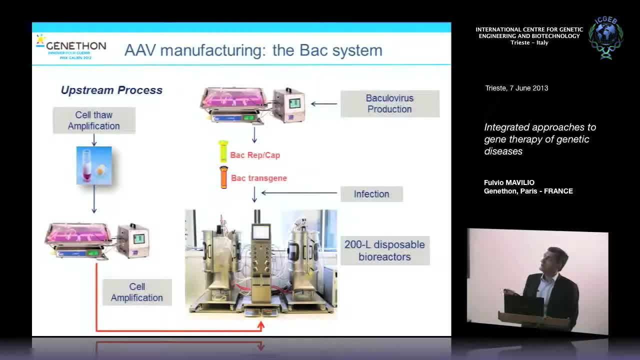 the other that calls for the transgene, in our case the u7. these two viruses are produced in sf9 cells, in bioreactors, essentially through one, a number of steps, but the bottom line is that you can use industry type of technology with this. Sartorius, big boys of. 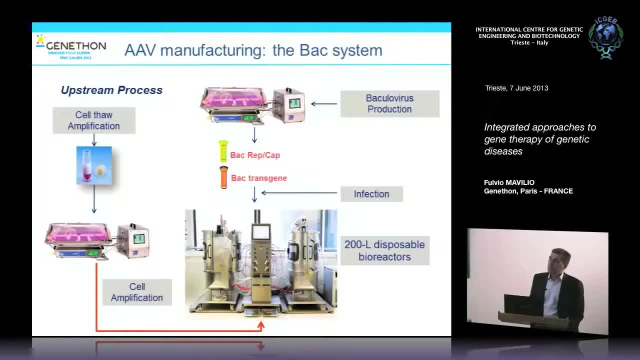 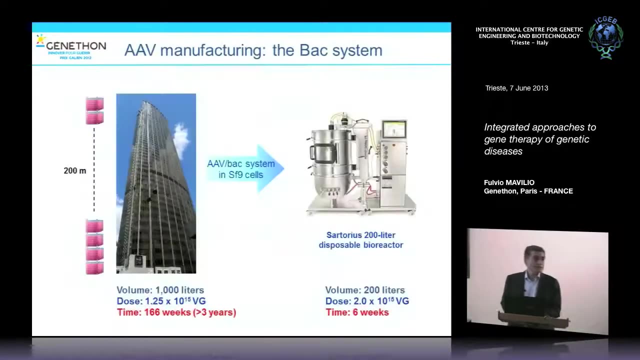 Sartorius, big boys of twin of 200 liters each. bioreactors that produce very high doses of AAV in GMP, ready for clinical use. so this is the type of stuff that we use for dogs. and just to give you an idea why this is important, to produce the dose of AAV 8. 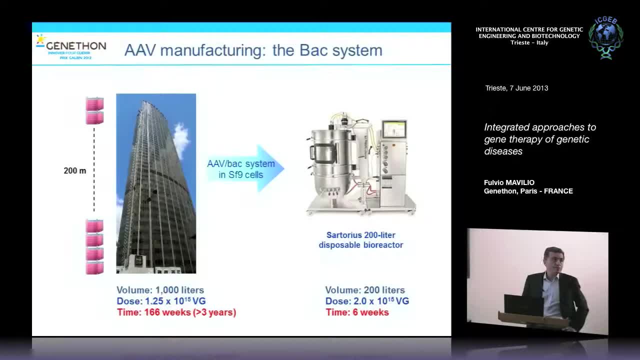 that is necessary to treat the first cohort of 30 patients, which is the clinical trials that it is planned by Geneton and the Institute of Biology in Paris. we would essentially need 1000 liters of culture with the standard cell Factory based transfection technology, which is a pile of almost 200. 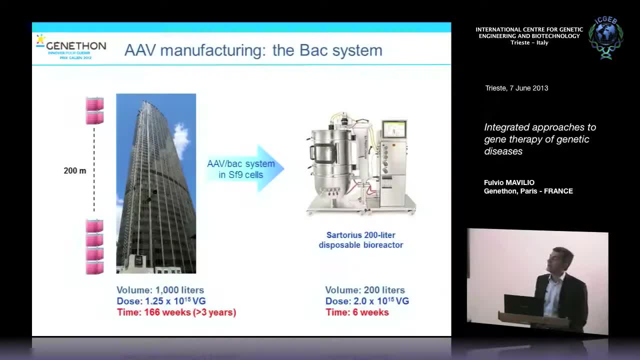 meters. this is the, a toolmanджana in the center of Paris, which is 200 meters, and the time that he takes to produce this is approximately three years. you can do exactly the same things in one run of 200 liters with basil and one by a. 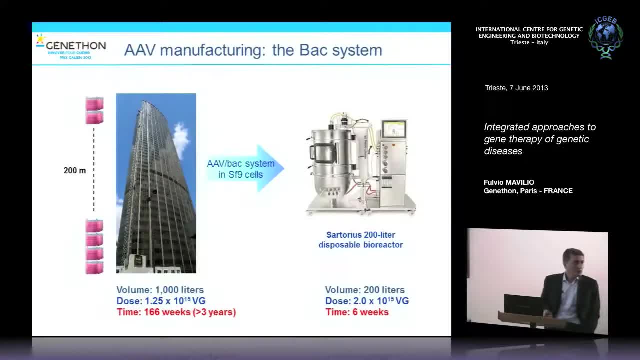 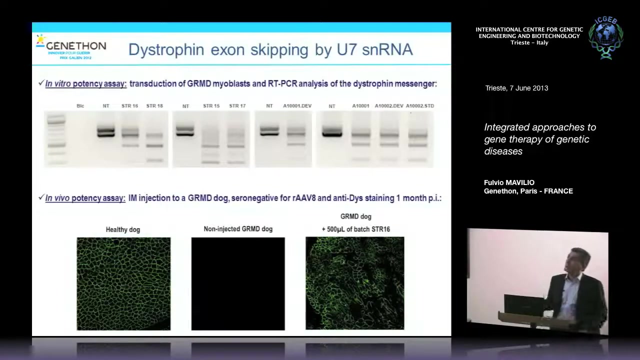 and produce essentially the same dose in six weeks. So this is the type of technological upgrade in the production of these things that makes a difference between something that is theoretically feasible but practically almost impossible and something that can be done. Going back to science, this essentially shows that in the dogs, 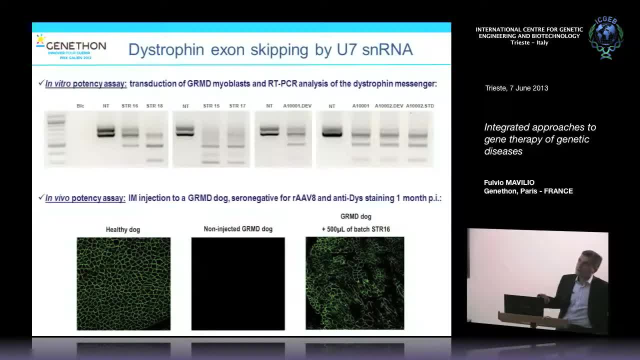 the exonskipping can work in untreated and untreated muscles. These are muscle biopsies. I'm sorry, this is the in vitro potency acids. These essentially, are myoblasts taken by the dog. This is an in vivo potency acid. 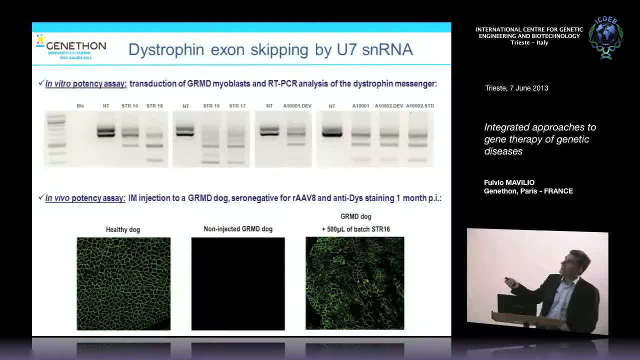 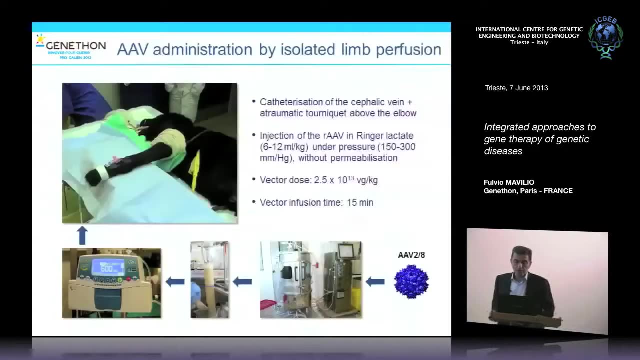 It shows exactly the same thing, But you can see here these are the skipped RNAs and these are the unskipped RNAs. This is essentially bottom line, dose dependent and unskipped, And works: Higher dose- higher skipping. Lower dose- lower skipping. 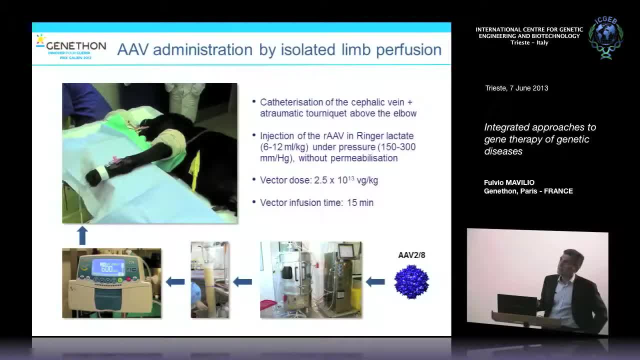 This can be done in dogs. as I said, The AAV is injected by a technology that's called isolated limb perfusion. It's essentially a tourniquet that you apply to the forward limb of one of these pure animals. This is not the GMD dogs. 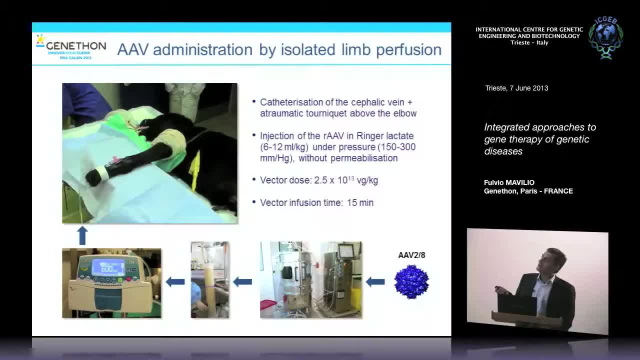 It's another type of dogs that I will show you in 10 minutes, But it's essentially the same technology. You can essentially use a pump to apply the AAV into the circulation, into this limb that is blocked with a certain pressure, a certain flow rate. 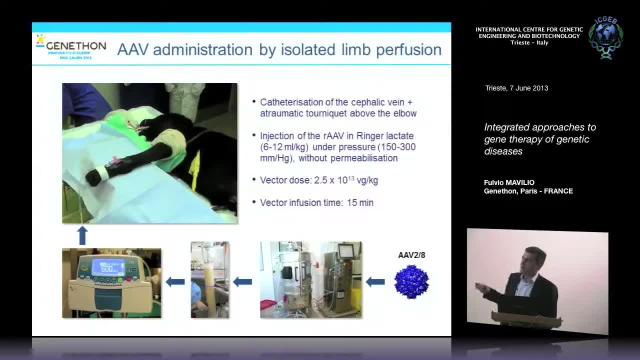 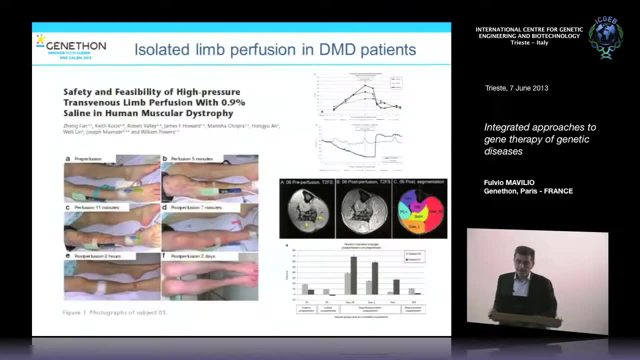 Everything has been standardized And the vector comes from the process that I described. that includes purification and affinity columns. Whoever is interested in this, I can give you details after my presentation. So this is injected in the dog And, of course, just to let you know. 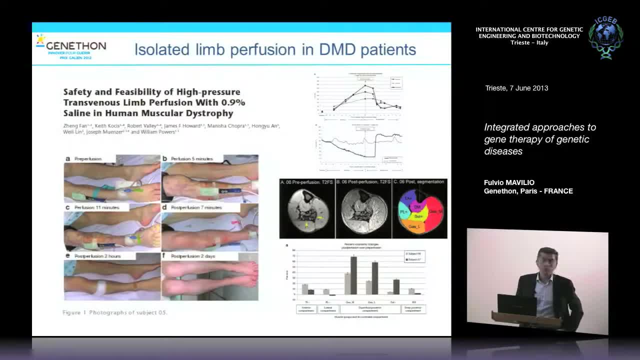 this is a technology that is completely usable in patients And actually it's even published a clinical trial in volunteers. volunteer patients of Duchenne has been injected with saline And just to show that this is possible, that of course the leg swells quite a bit. 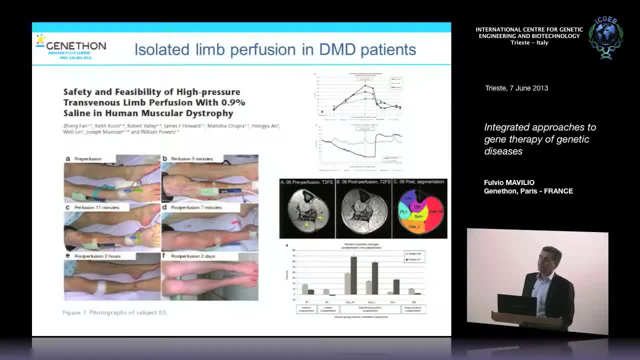 The volume that is injected is very significant but very rapidly goes back to normal volume and with zero complications for the patient. So this is practically feasible. This is the route of administration that we will follow in our patients: injecting virus and not salted water. 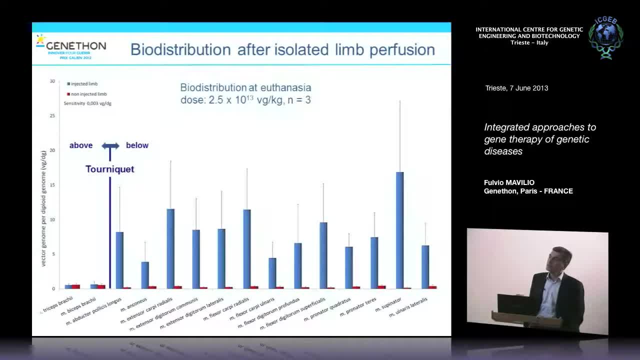 The tourniquet. if you are good at doing this, if you are a good surgeon, works relatively well. This is the biodistributor. This is the distribution of the vector in the muscles below the tourniquet and above the tourniquet. 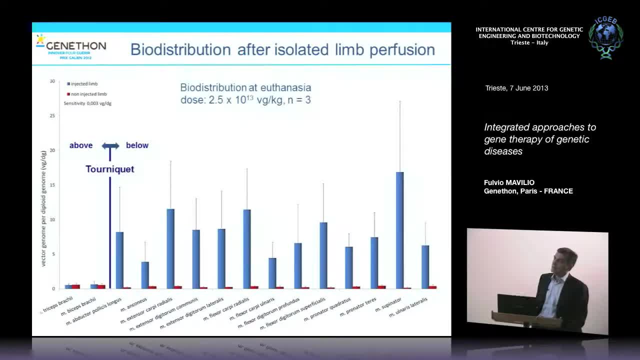 or the contralateral legs And, as you can see, most of the all the muscles in the injected leg are transduced with a variable vector copy number. The dose that has been administered is 2.510 to the 13 VGBRK. 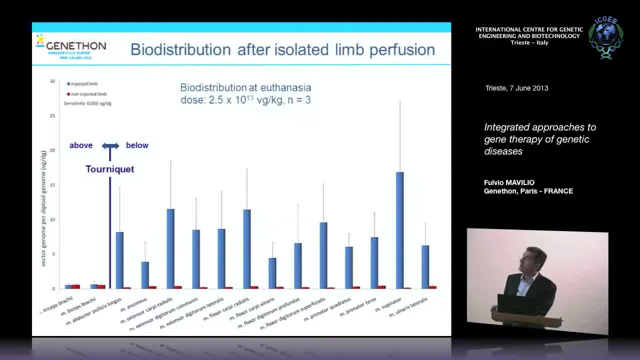 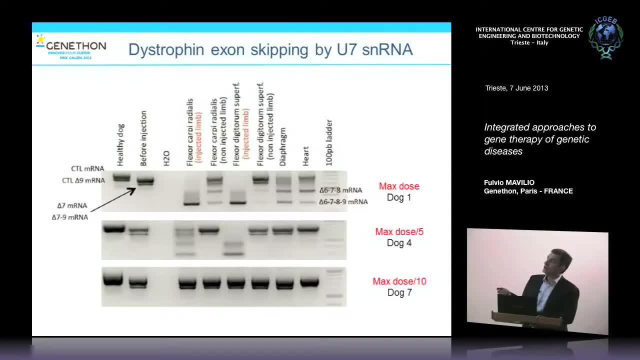 which is a very significant dose. as you may understand, This shows that the exon skipping occurs in vivo. At the maximum dose, you have a very efficient skipping. At one-fifth of the dose, you have skipping, but less efficiency. 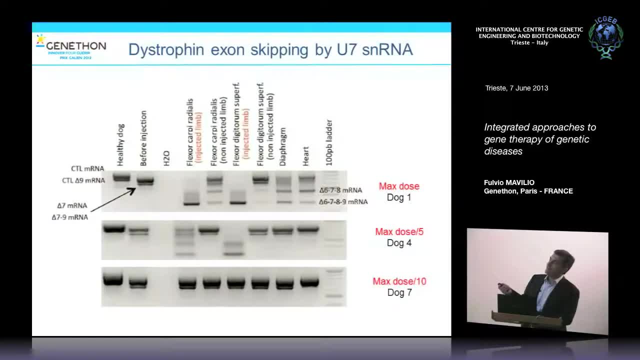 And in some tissues this doesn't happen. Of course, the more you apply, the more you leak into the rest of the body. So, not surprisingly, for the maximal dose we have transduction of the heart, the diaphragm. 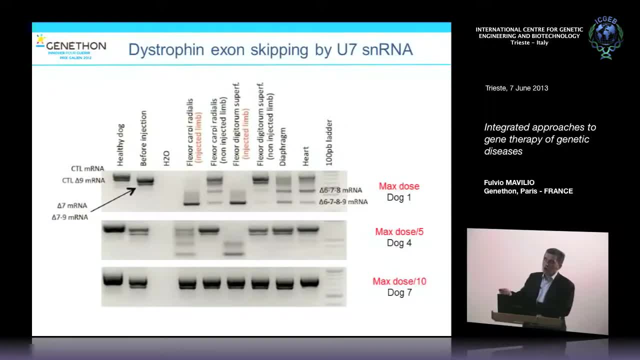 and other muscles And when you reduce the dose, essentially only the injected leg is transduced. It skips the exon One-tenth of the dose. you start losing the exon skipping. So this is dose dependent and finding the dose is crucial. 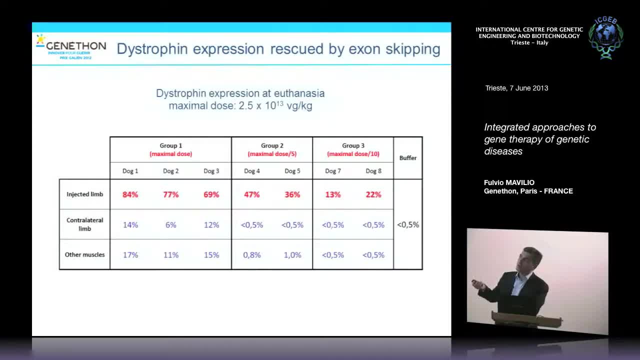 This shows the same thing at the level of percentage of fibers expressing dystrophy. Maximal dose: you have expression in the contralateral lip or in other muscles. One-fifth of the dose is essentially restricted to the injected lip. One-tenth of the dose. 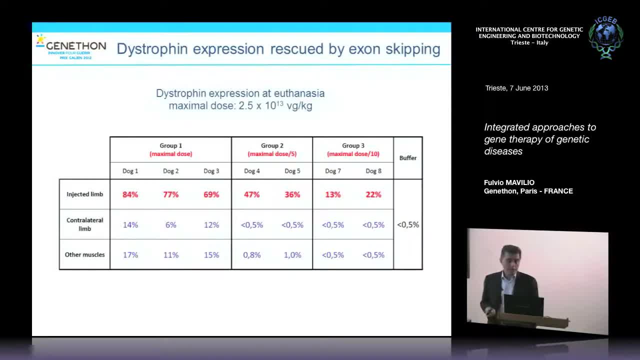 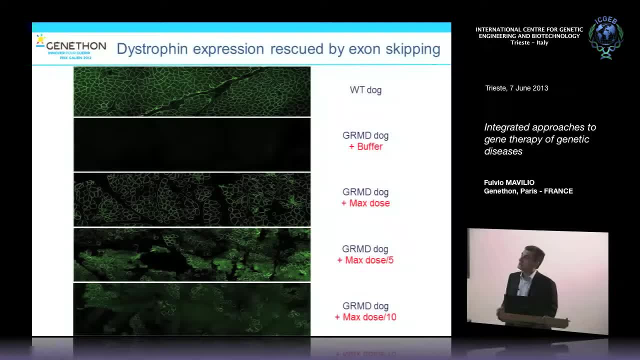 you go beyond the percentage of fibers that are, you know, therapeutic. So this is the dose that you need to use, at least in the dog. This gives you an idea. It doesn't show very well, but essentially, transduction is very efficient. 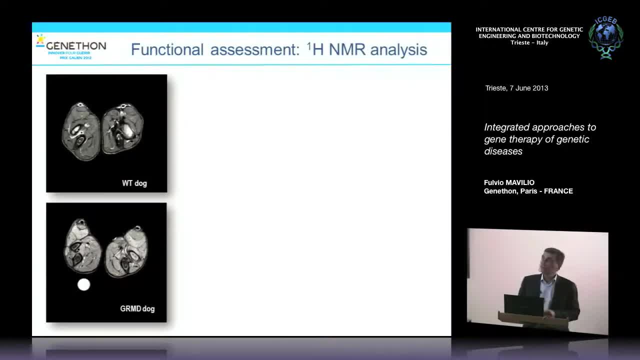 I'll show you some examples of functional tests that are done on these dogs, which I think is interesting. I'm actually fascinated by how many things you can do in dogs that you can do in patients and you can essentially test in dogs. One of this is NMR. 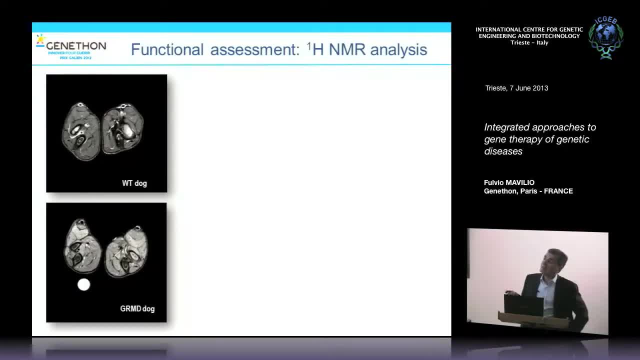 So by doing this proton NMR analysis, this is sort of a functional in vivo, non-invasive test, And when you do an NMR on the muscle of a normal dog, this is the type of pattern that you get. This is a transvex section. 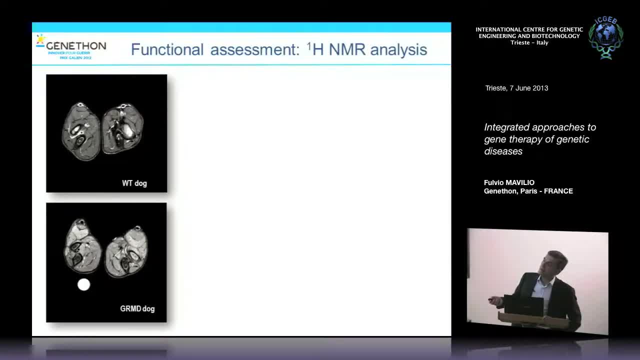 if I can say this, In a dystrophic dog you have this, this very strong white signal that essentially shows that the metabolism there is completely altered, and you have a signal that you're not supposed to have in the normal musculature. 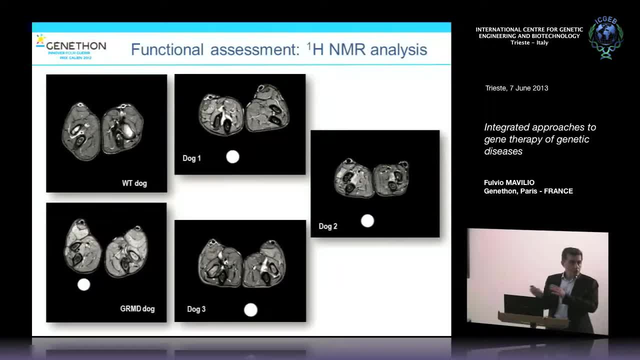 And you can use the same type of readout which is transposable to humans. Actually, this is a clinical NMR machine to look at what happens in the treated dogs And, as you see, the treated legs of dog one, two and three. 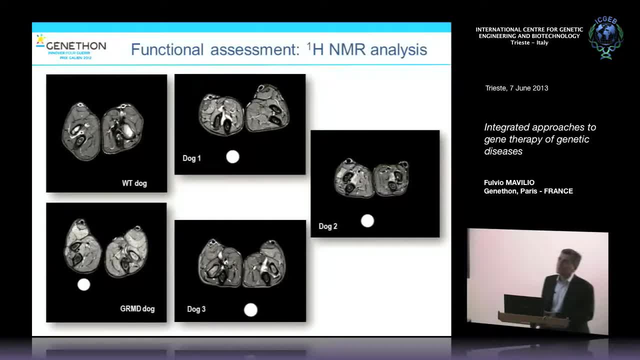 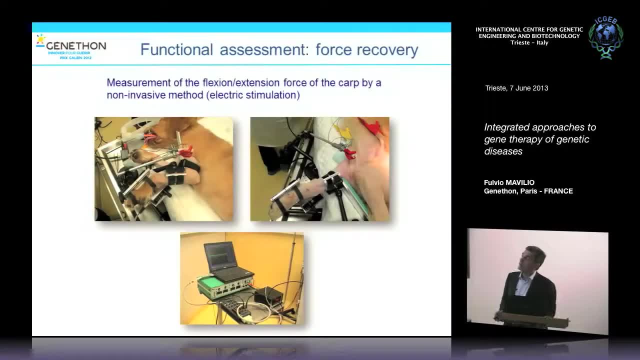 is essentially have essentially a pattern that is reminiscent of a normal animals and not of the dystrophic animal. A second readout that is also very useful, is important and very relevant in terms of clinical reconstitutional function is, of course, forced recovery. So in this, dogs. 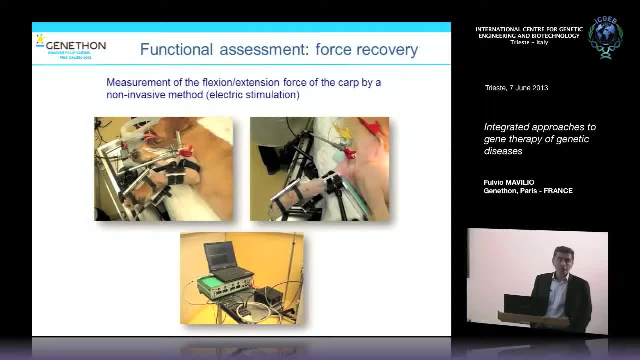 which are injected relatively early in the course of the disease, so they're approximately at three months of age. you can measure. the dog here is in under anesthesia and the measurement is done by inducing contraction by electric stimulation, And there are machines that have been developed. 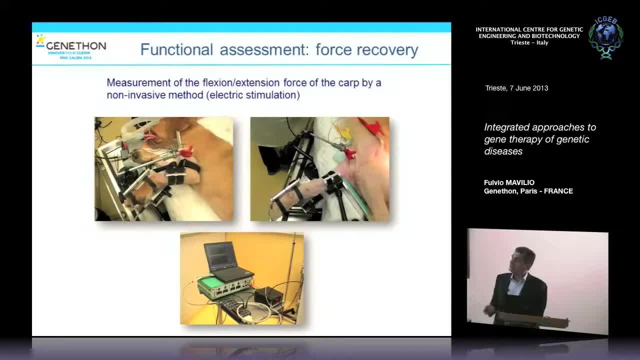 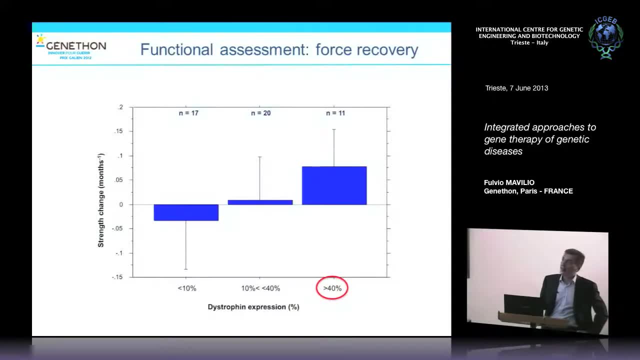 that can essentially measure force, contraction, induced force, And this is, I think, an interesting piece of results that are obtained in these animals, because if this is the type of results that you get in, and the numbers here, as you see, are significant- 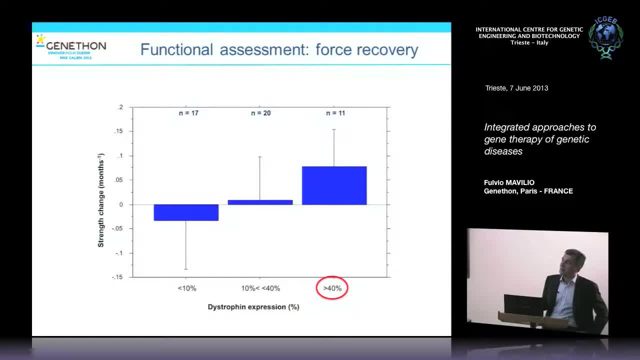 many dogs have been treated in this preclinical assay. If you have less than 10% of the dystrophy positive fibers, essentially you have no effect. The dystrophy progresses, the dog doesn't recover any force and this is, this is the result. 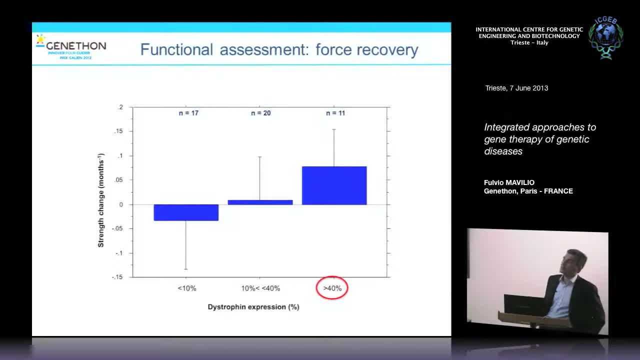 This is what you have if you have between 10, 40% of dystrophin expressing fibers, And this is what you get when you go above 40% of dystrophin positive fibers. This type of assay allows to predict that, in order to be 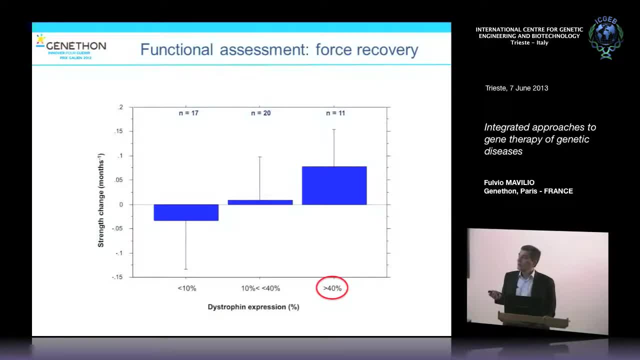 to reach therapeutic levels of dystrophin expression, certainly in dogs, most likely in patients. this is the level that you have to achieve, So the threshold is very high. You have to achieve at least 40% of the fibers in the target muscle. 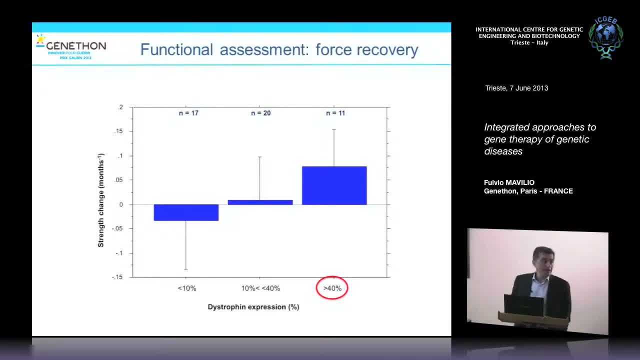 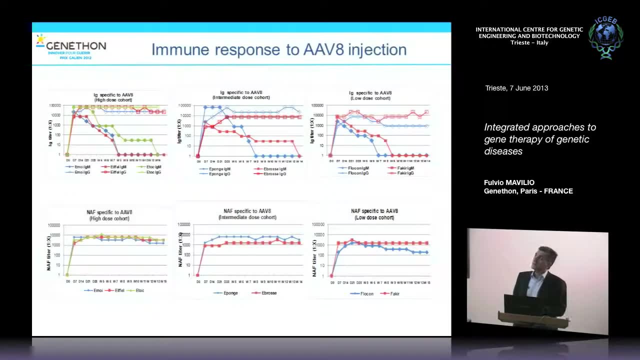 in order to stop dystrophin progression and to essentially have a benefit in terms of recovery of force. For those of you that are interested in immunology, I'm going very fast because otherwise I will never finish today The injection of AV8, of course. 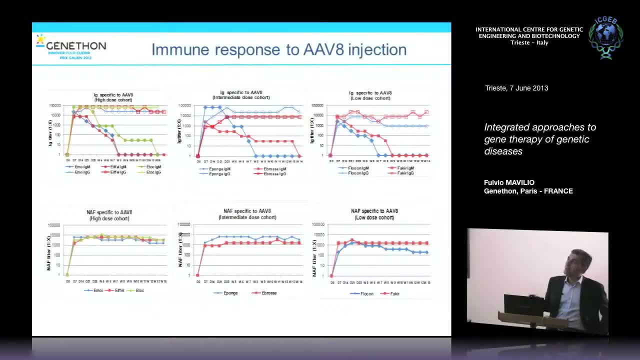 these dogs are naive for AV8,, of course causes and the appearance of neutralizing antibodies and neutralizing activity in the serum against AV8,. almost immediately after injection The IgG response is persistent. The other responses are not. Again, I won't go into the details, but essentially, 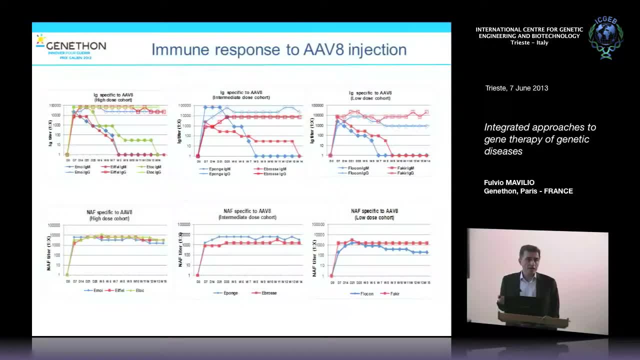 this is not something that you can repeat, And this is another challenge of this type of therapies in humans. You have to realize that once you reach this type of level of specific neutralizing activity in the serum, there's no way you're going to re-inject again. 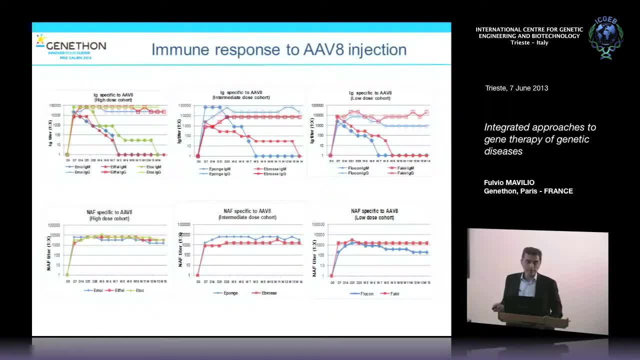 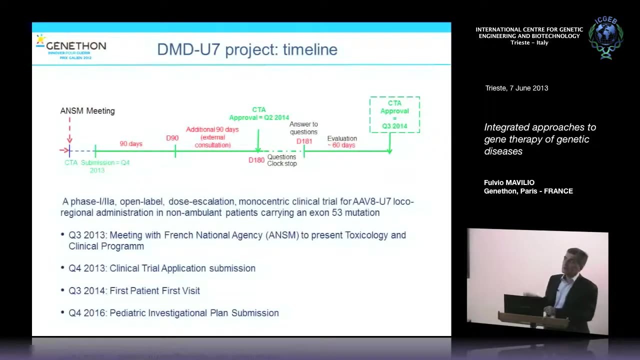 the same serotype in a dog, in a monkey or in a patient. So in planning clinical trials you have to take into account that you will not have the luxury of repeating the type of treatment in the same patient. Just to give you an idea of this story. 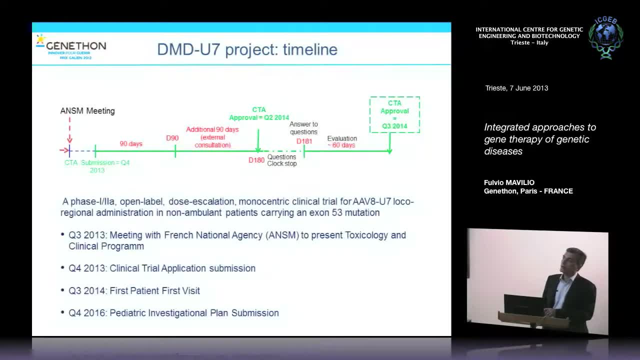 as you understand, it started many years ago and it's going progressively towards a clinical trial. We are approximately here with the clinical protocol ready, a natural history study done, a number of things done, the GMP production already done. We do expect, we do hope to be able to treat patients. 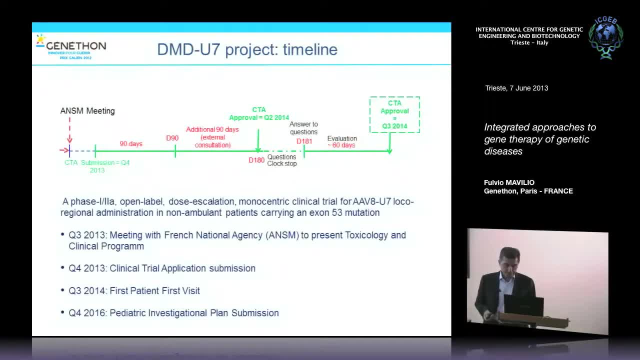 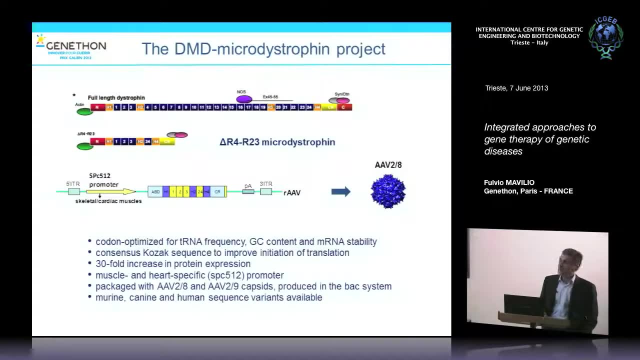 and we hope to be able to treat patients, and we hope to be able to treat patients, and we hope to be able to treat patients at the end of next year. Just to give you a clue of what are the alternatives. of course, as I said, skipping exo53 sounds interesting. 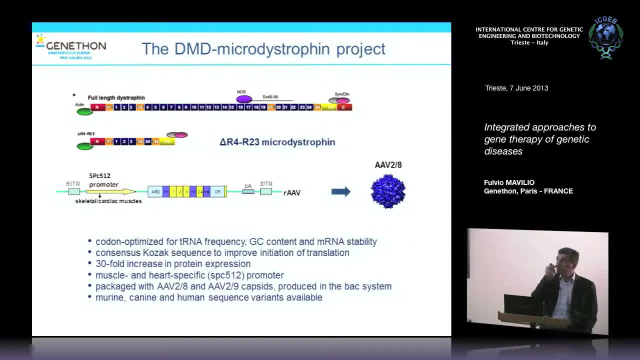 but it's less than 10% of the patients. what you do with the rest of the patients? Of course you can theoretically think of devising exon skipping molecules for almost any exons. but certainly you can't do much if you have a large gene deletion. 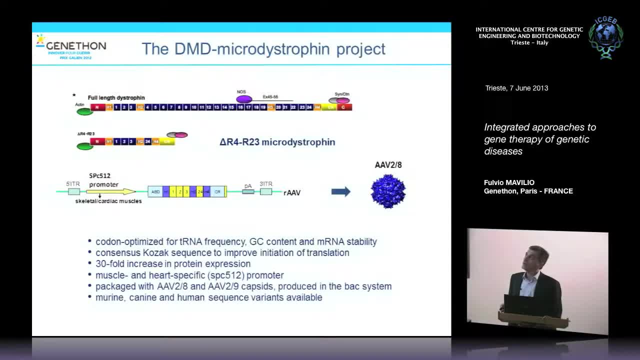 which accounts for more than one third of the of the exons, of the exons of the exons. So no way to try and get a duplicate product of the exons. has to do with mutations in humans And I'm not sure that it would be. 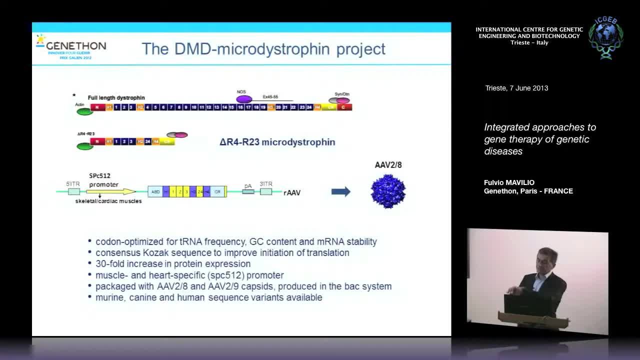 practically feasible to design exon skipping strategies for everything, So there are other possible strategies. as I said, the gene is very big but the cDNA is huge and it can not be possibly put into an AAV. Years ago, Jeff Chamberlain and George Dixon designed a number of molecules that essentially 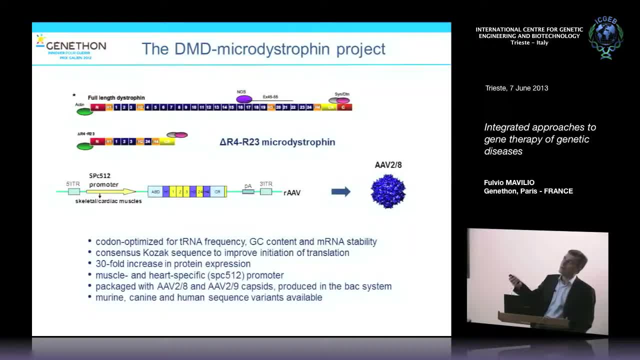 are completely, very much reduced and almost completely devoid of the internal rod domain. They only have the terminal C terminal and a few exons of the rod domain. So these are called micro dystrophins or mini dystrophins and they essentially work, even if it reduced efficiency with respect to the normal molecule. 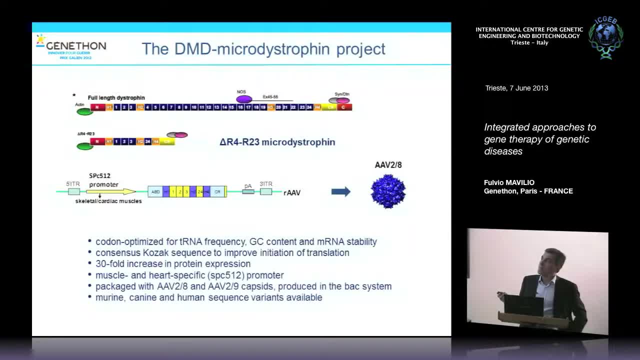 Now this thing can be put into a vector. So, essentially, what I will show you in the next slides is what you can restore, in terms of all the parameters that I showed you before, by using a synthetic promoter, a muscle specific strong promoter, and this small RNA coding for this micro dystrophin over here. 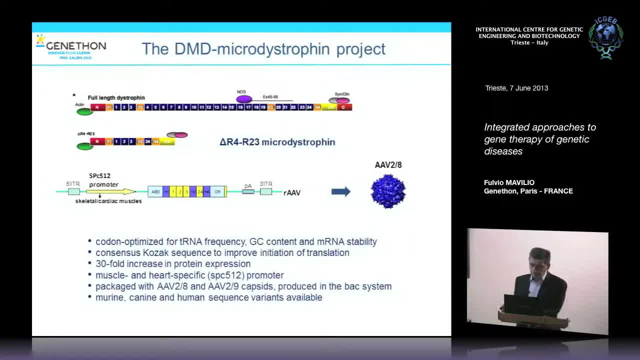 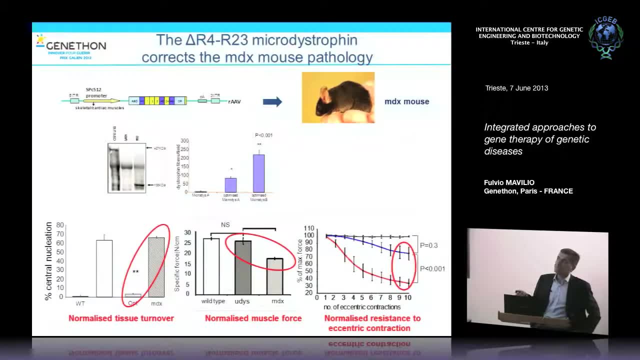 Again, the serotype is small, It's 2.8.. And a few years ago George Dixon showed that in the MDX mouse this protein works very well. This is the size of the protein. compared to the normal dystrophin, It's really much smaller. 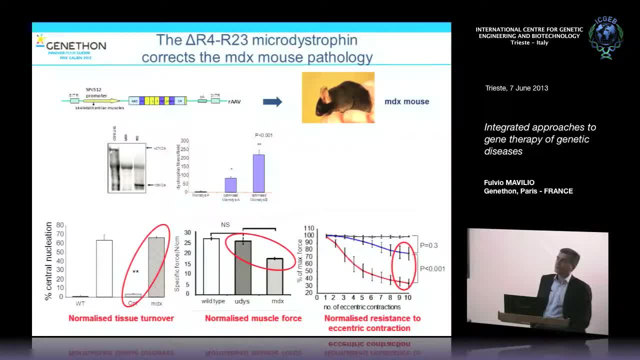 And you can normalize tissue turnover, reverse the dystrophic phenotype in the MDX, normalize muscle force, normalize resistance to eccentric contraction, a number of parameters. So in the mouse This works. But I must say that almost everything works in the mouse. 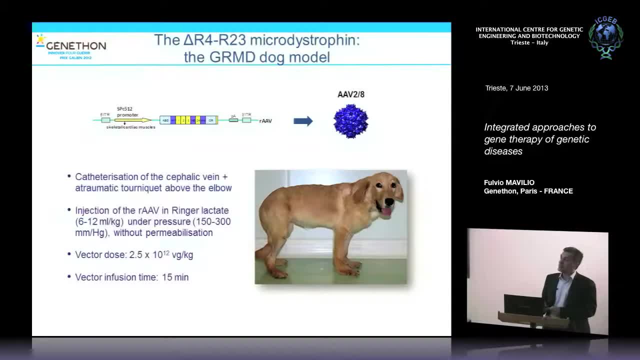 So what happens when you put this in the dog? The dog is much more challenging. So we decided to use the same dog and this experiment started last year, So they're relatively recent. Nothing is published. We started with a vector dose that is one-tenth of what we use for the exon, skipping based. 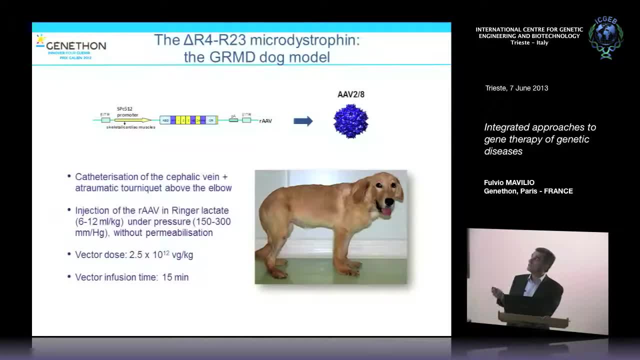 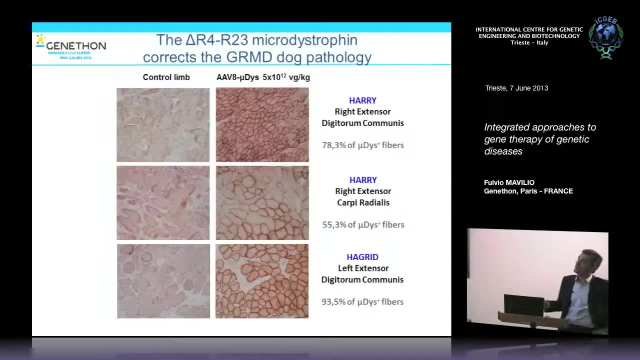 on in vitro assay that shows that essentially, this, This vector, is more efficient. Producing protein is more efficient than skipping exon And essentially, the dog went through the very same procedure And this is the type of results. So these are three dogs that have been injected local, regionally. 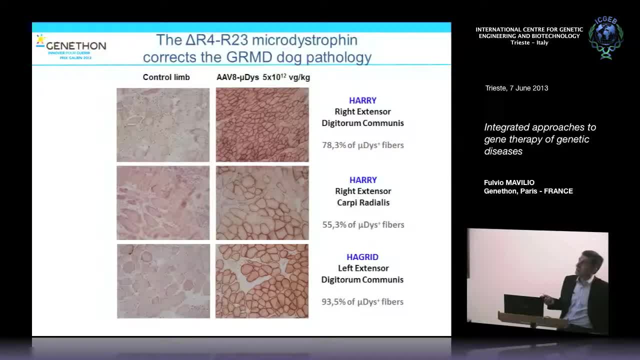 And these are three muscle, actually two dogs in three different muscles. And, as you see, as you can see here, the percentage of fibers that are positive for dystrophinism they're very low. The percentage for dystrophin in these animals is very, very high. 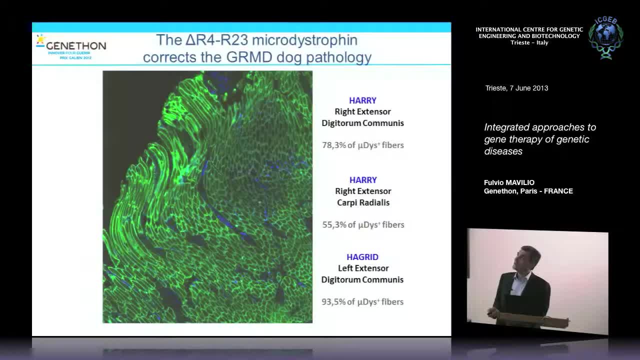 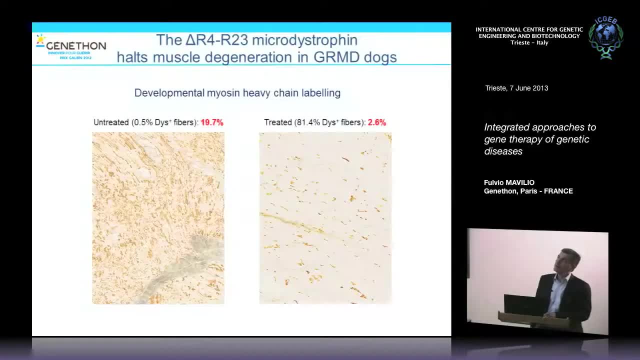 And this is just to give you an idea- by immunofluorescence, which makes a nicer picture. A number of parameters show that this is functionally relevant. Developmental myosin heavy chain is something that labels fibers when the turnover is very. 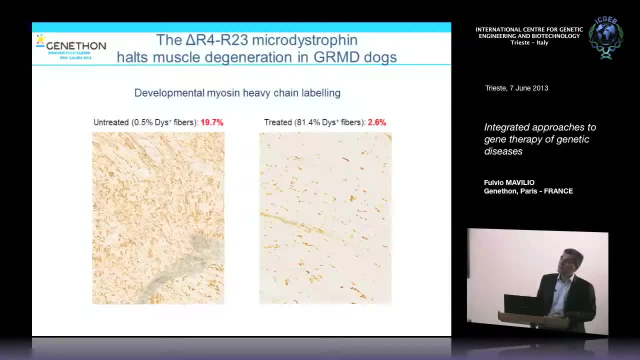 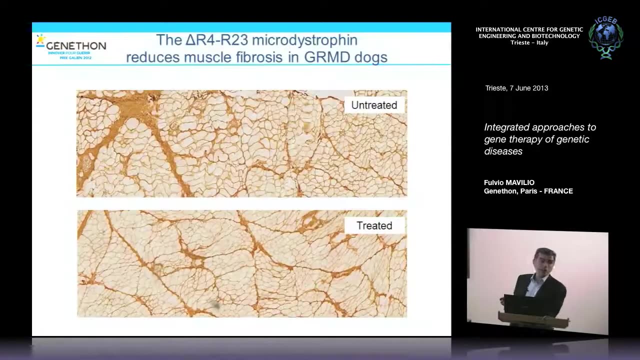 high. So when you have a lot of labeling means that these fibers are dying and are regenerated. very often After treatment this turnover goes down to 2% rather than 20%. So very good data. Fibrosis, which in the dog is part of the phenotype, is very much reduced. 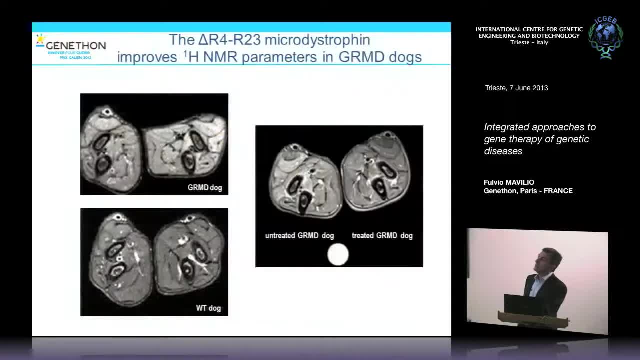 And this is just a qualitative assessment of this- NMR spectroscopy gives the same type of results. So, again, the treated muscle look much more like the wild type, dystrophic, And this is the result, And this is the result. This is the bones on the bones. 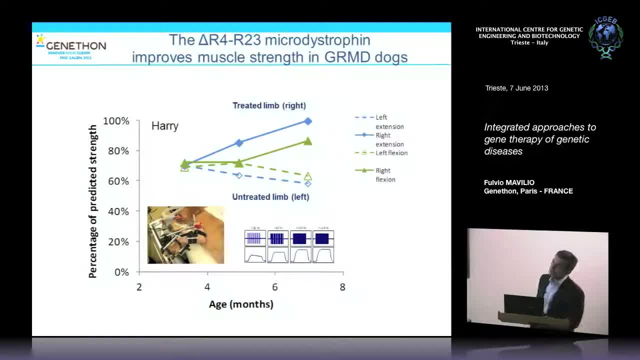 So this is the normal muscle And in terms of a percentage of predicted strength that is recovered, so strength increases in this treated animal. these are the untreated, these are the treated limbs in the same animal And this is very significant. And this we are talking about experiments done up to eight months after infusion. 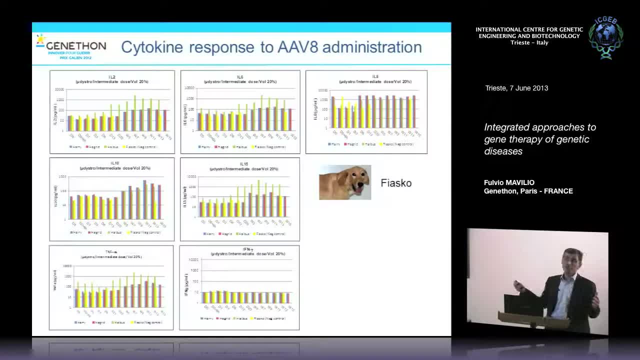 And the immunology. this is also important because here we are expressing, if you wish, an artificial protein, and the issue whether this can cause rejection is a crucial issue. These are all cytokines that essentially show that the response is not particularly predictive. 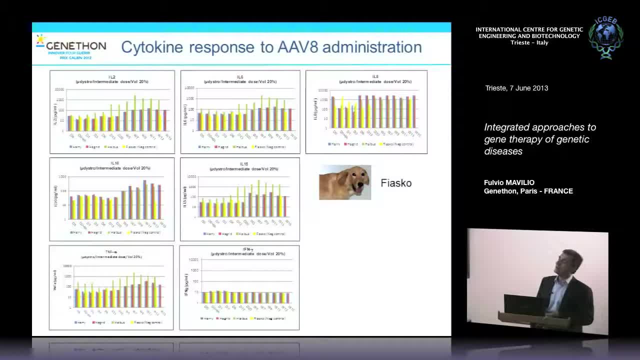 in this animal. So Fiasco is an untreated animal which is in yellow in all these things, And the treated animal, with the exception of one, essentially show the same pattern. Treated animal are these three. Besides learning French, I had to learn also who are these guys here and honestly, I didn't. 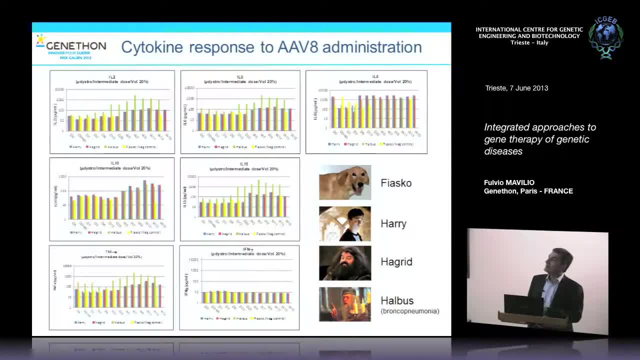 know them before, But the kids that are working with dogs use names that are very romantic. Anyway, the only one that showed some cytokine response was this old guy here, Halbus, But he had Bronchopneumonia, So most likely that's an inflammatory response not caused by the vector. 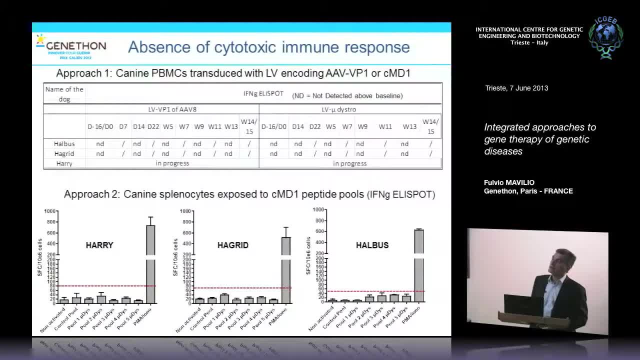 And, most importantly, by two different approaches. there is no evidence of cytotoxic T cell mediated immune response against the fibers, which is the most important thing as far as we are concerned. I don't have the time to show you this data, so you need to believe me. 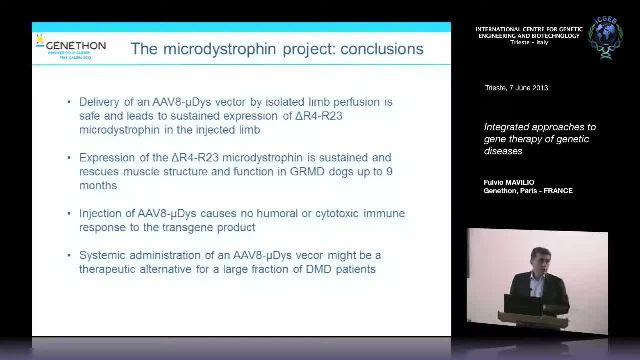 So, just to conclude, there are two approaches that we can use to treat muscle. One is very close to the clinics, which is the exon, skipping This other one that is going very fast and, honestly, I think, very promising. The difference is that, theoretically, a micro dystrophy can be used in any patient. 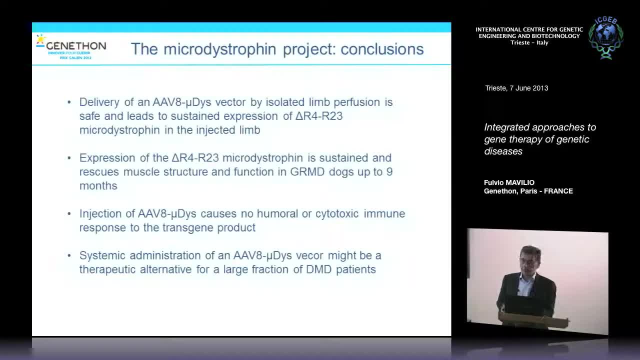 And exon skipping is limited to patients, the exons that can be skipped. I don't have particularly preference for one or the other approach. I think that only clinical trials will tell us Whether or not this has a chance to be beneficial in this little patients. 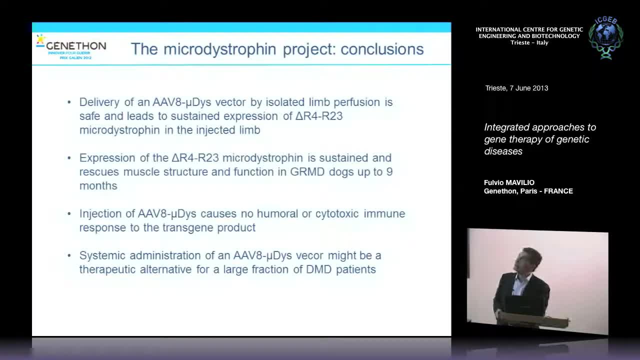 So let me spend the last 20 minutes or so by giving you an idea of at least another model of neuromuscular disease, and then what we are doing in the blood disease is that, as I told you, is the second big part of what we are doing. 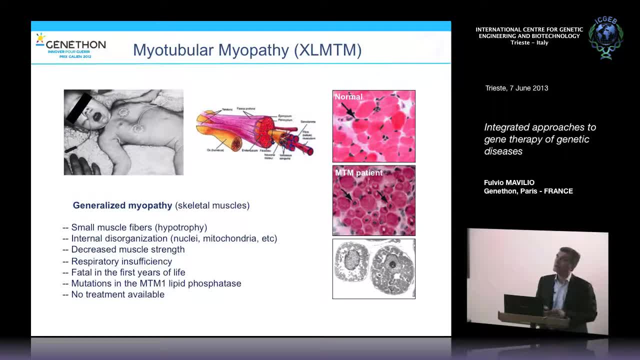 This other disease which very few people know. it's extremely rare. it's called myotubular myopathy. It's an interesting disease because it's not a dystrophy which gives us the hope that these patients can be treated. It's a deficiency of an enzyme which is called MTM1.. 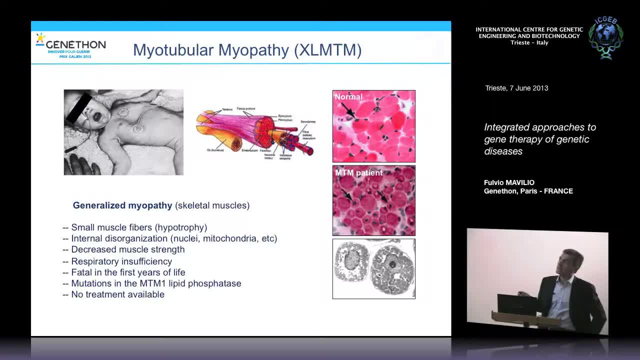 It's a lipid phosphatase. It's very crucial to muscle function. In the absence of this enzyme, Well, Patients essentially die. So now, patients don't survive the second year of life, Essentially die by complete respiratory failure. Those with residual protein levels survive longer, but they have zero motor function and they normally go into ventilation, assisted ventilation, at the age of three, four. So it's an extremely severe disease. Survival is life-explanatory. Life expectancy does not exceed ten years in the best cases. The fibers, the muscle essentially does not develop and does not contract. 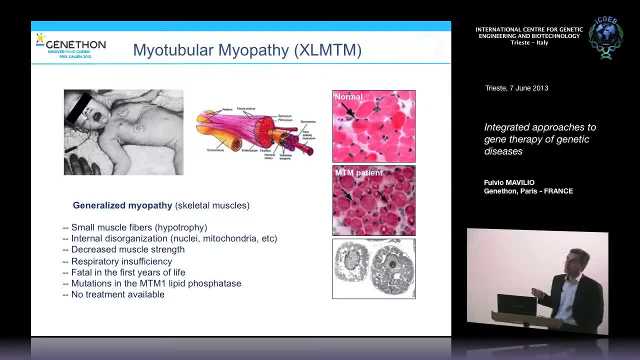 So it's there. It's not a dystrophic muscle, So it does not degenerate. It's simply not working well because of the absence of this enzyme. And as a very characteristic phenotype, it's the central nucleation of very small fibers. 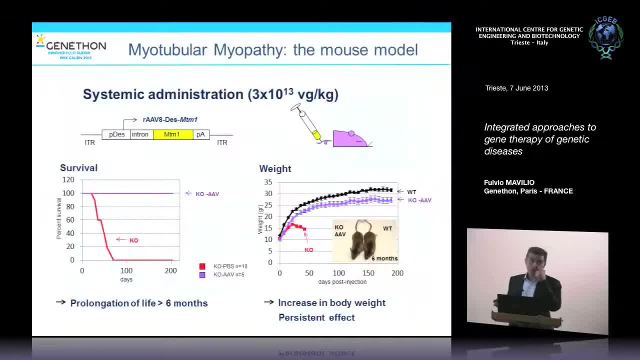 To make a long story short, I'm sorry. I'm sorry, It's a long story short. Anna Bush-Bellot, a scientist at Ingenidon, a few years ago developed a mouse model, Actually more than one, And I don't have the time to show you all the genetics of this assay, which is extremely. 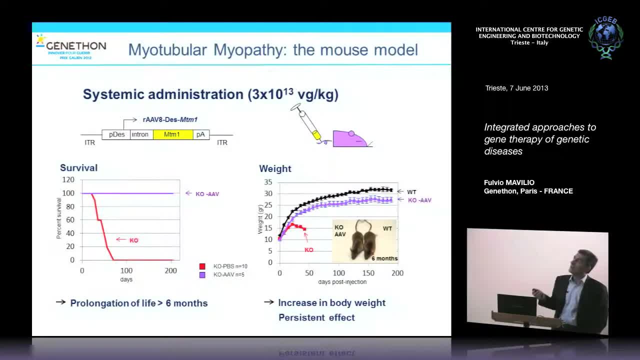 interesting and just showing one of these models. This is a knockout And essentially the red line. this is how the mice behave. The mouse reproduces very well the human phenotype. These mice are severely impaired in their skeletal muscle function. They all die very soon. 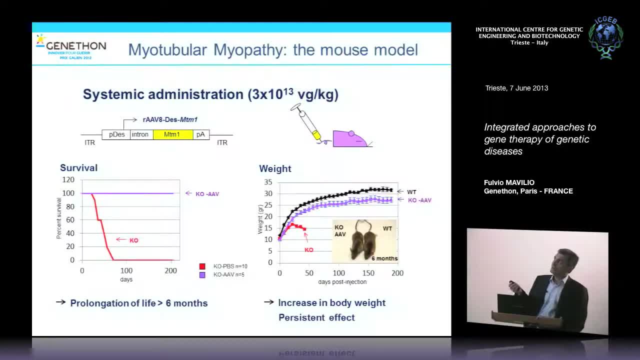 If you give a tail vein injection of this dose of AV8 encoding MTM1 under the Desmin promoter, which is muscle specific, you rescue 100% of the animals. Not only you rescue these animals, but you can rescue these animals even if you inject here. 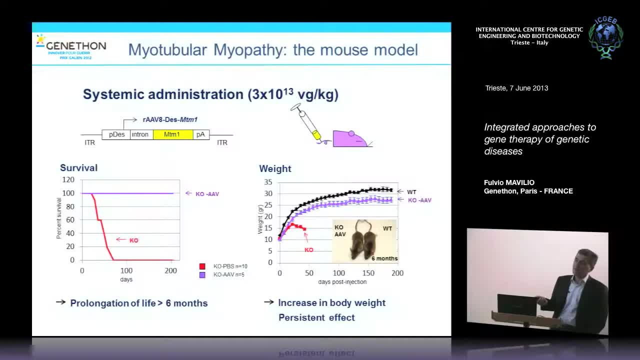 So not only you can prevent the disease by injecting in the first two weeks of life, but you can stop progression and rescue completely the animals if you inject later, when the disease has already started. This is WAIT. This is the wild type animal. This is the knockout treated with AV. 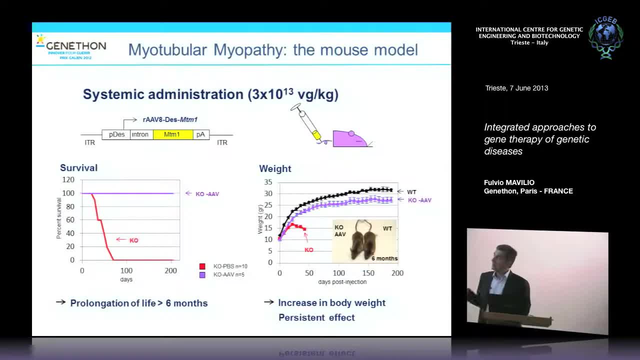 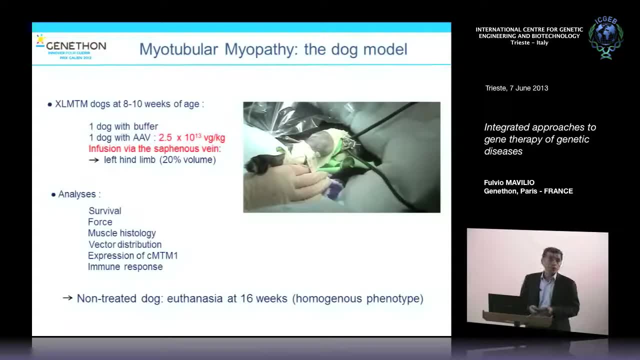 This is the knockout untreated. I don't need to explain that this is a complete cure in the animal For this disease there exists. This is a dog model And it's now at the University of Washington in Seattle. This is the group of Casey Childers. 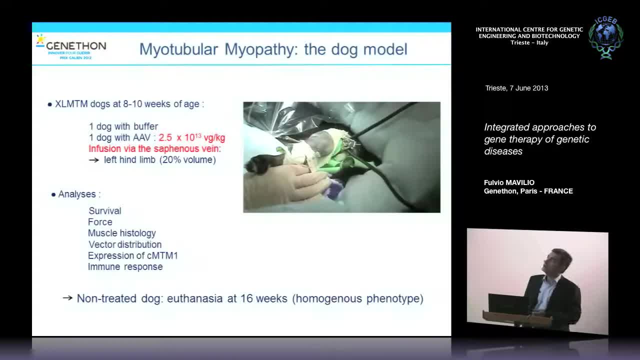 that work with these animals, And when Anna started the collaboration with them, they essentially put together everything we already know about isolated limb perfusion in these Labrador dogs. These are black dogs, the one that you have seen before. So, again, we essentially did the same thing. 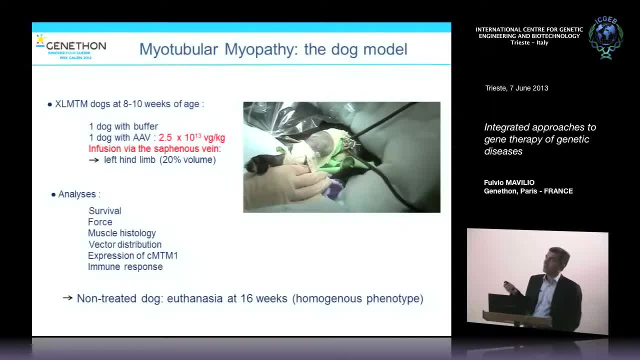 This is an AV8 producer. It's produced in Baculo. that expresses MTM1 under the lesbian promoter, And what you assess in these animals is here. The non-treated dogs have to be euthanized before 16 weeks. They don't survive. 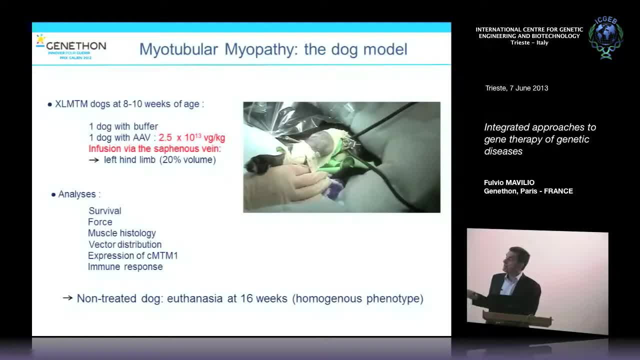 I will show you the phenotype in a moment. And this is very homogeneous. They all die. Well, actually, you have to euthanize them, OK. And the question here was: can we rescue muscle function by this type of injection? 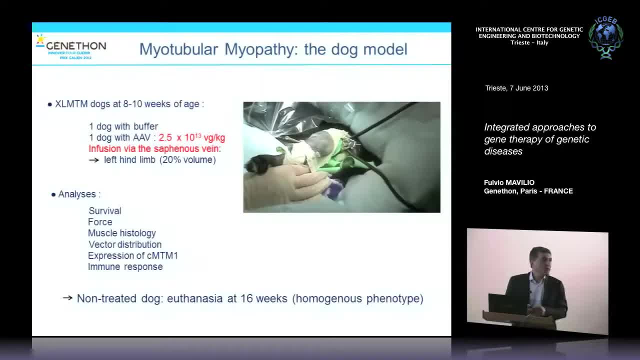 Fortunately for us, the Americans are not very good at applying tourniquets. So, as you will see in a moment, this isolated limb perfusion turned out to be not very isolated And we essentially injected almost systemically this dose. Many of this went into one leg. But after 10 minutes you release the tourniquet and whatever is left goes around. Before giving you the idea of the blood program, let me acknowledge the gigantic group of people that is doing all this research. It's half of genital, basically. 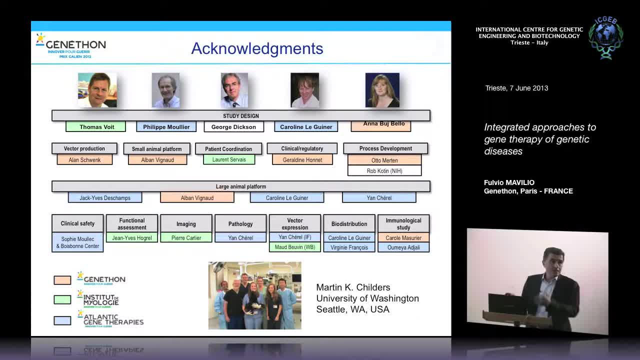 Let me acknowledge Thomas Voigt. He's the director of the Institute of Myology. the clinics in which this is done, where all the physicians are, where the patients are treated, where the gene therapy trial will be, It will be done. 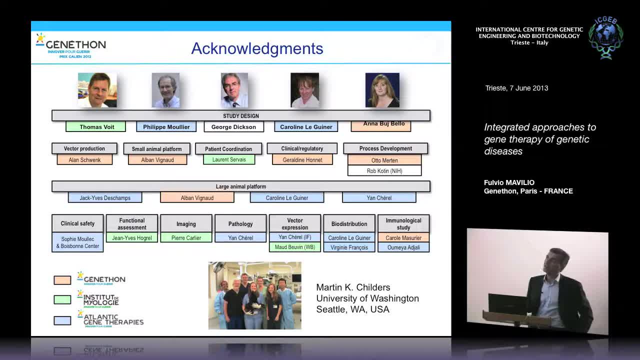 Philippe Moullier was the scientific director of genital for a little less than two years before I came And he's still the PI in the exon skipping study. George Dixon is at UCL in London and he's the PI of the micro dystrophin study. 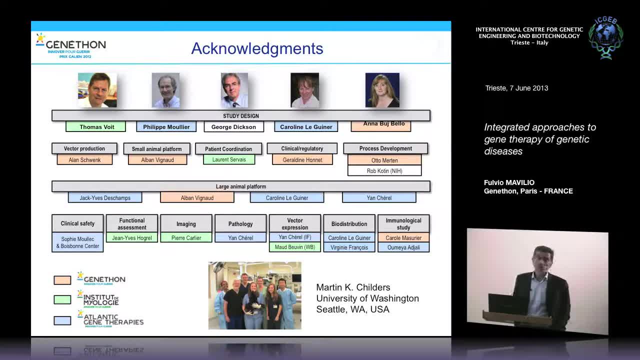 Caroline Leguinet and Nant works with the dystrophic dogs And Anna Busch-Pellot works with the myopathy project- OK, And she's the project leader And the group of Casey Childers in Seattle helped us for power off. 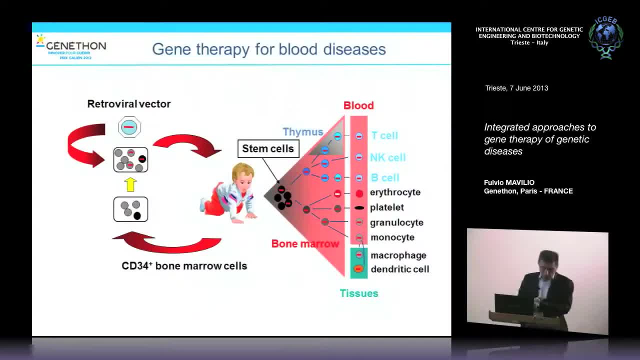 Oh no, With this So blood. Well, as you know, this is a completely different thing. So we don't inject viruses. It's not an AAV. We genetically manipulate stem cells and we inject genetically manipulated stem cells. 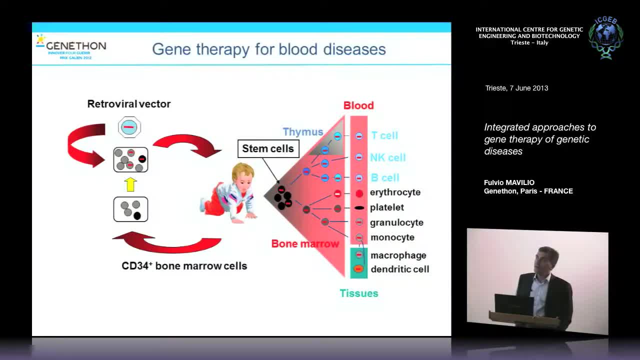 I'm sure that I don't have to tell you what this is. We use lentiviral vectors for transducing stem cells. This is the type of gene therapy that Mauro was kind enough to remind you. This is where the whole field started in early 90s. 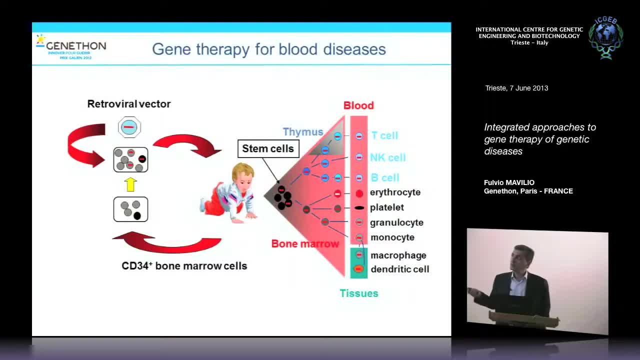 with adenosine deaminase deficiencies. Now there are many diseases that are treated essentially the same approach. You get C34 progenitor cells from the bone marrow or peripheral blood from patients. You transduce them in vitro with a retroviral vector. 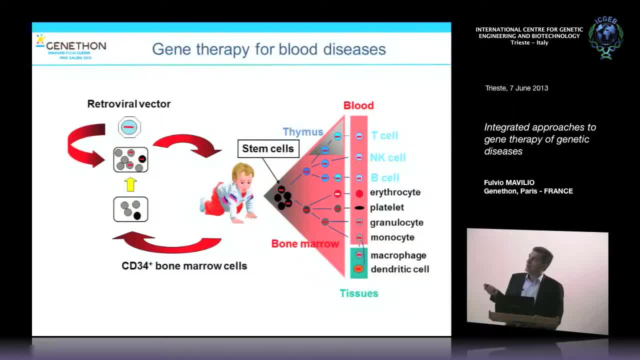 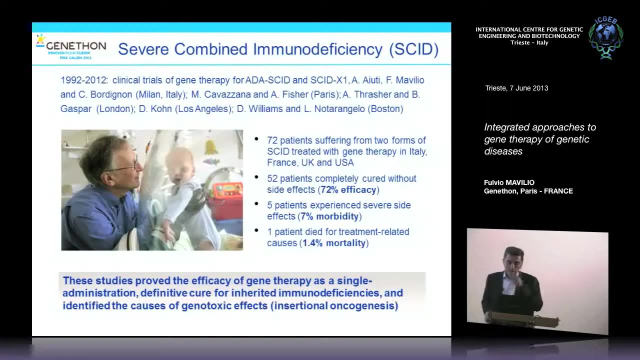 or lentiviral vectors whatever, And then you transplant them back into patients, with or without conditioning, And if you're good at transducing stem cells, you get gene transfer and gene expression in the lineages that you want to target. So I show you this slide to give you. 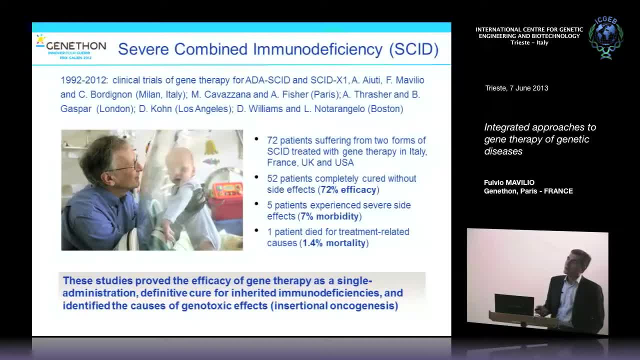 an idea of what in What many people think was a failure of gene therapy and essentially was the trials. there are many for severe combined immunodeficiency- Two types: ADA deficiency and common gamma receptor deficiency. Many groups were involved in this. 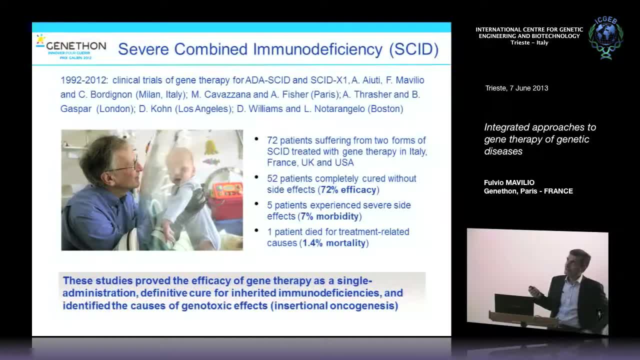 Our group in Milan at the time Marina Cavazzana and Alain Fischer. in Paris, Adrian Trascher and Bobby Gaspar in London, Dan Cohn in Los Angeles, David Williams and Gigi Rotarangelo in Boston, And all together since 1991, 72 patients have been treated. 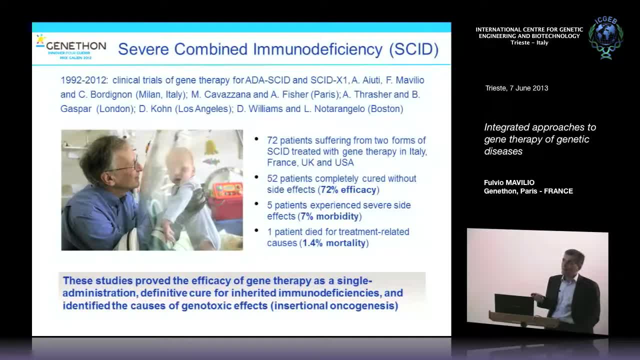 for all these type of diseases, and all with the same approach: retroviral vectors, not lentiviral vectors, coding for either the ADA gene or the X-KID gene. Now, nothing happened in the ADA gene. The patients were all cured. 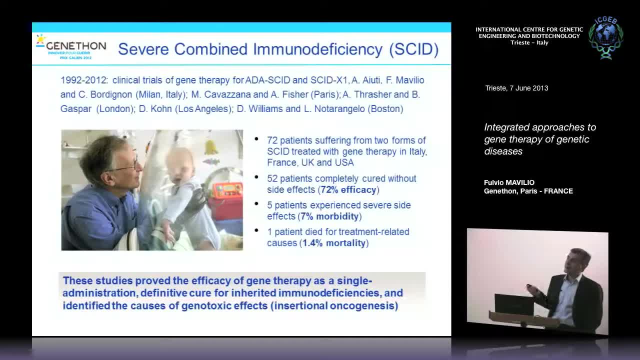 This was a clear history of success, But the other therapy is also a history of success, despite the sort of bad publicity that the occurrence of five leukemias due to insertion or oncogenesis caused in these patients. The numbers are here: 72 patients treated. 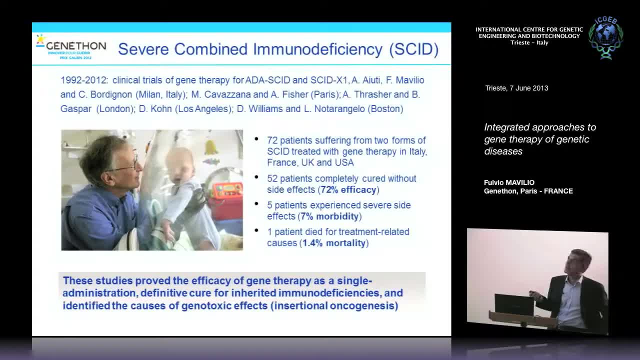 52 patients were completely cured. This is a lethal disease And these patients are alive and well, which is a 72% efficacy for a lethal disease, which is, I think, any therapy for any lethal disorders. with this type of numbers would be considered a fantastic. 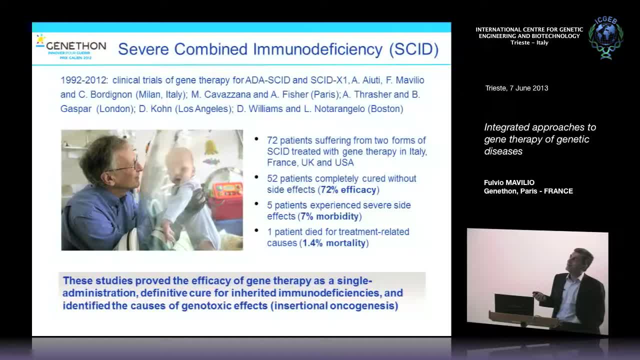 success in medicine And I think it is. Five patients experienced, As you probably know, leukemia due to insertion or oncogenesis, which is 7% morbidity if you consider all the patients. One patient died. The other four were treated and are still doing well. which is a mortality of 1.4.. The alternative for these patients, if they don't have a donor, is either die or have a mismatched bone marrow transplant, with a mortality between 25% and 45%. So this is the type of results that gene therapy shows. 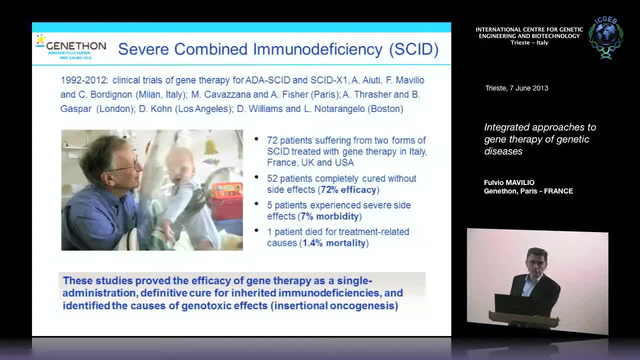 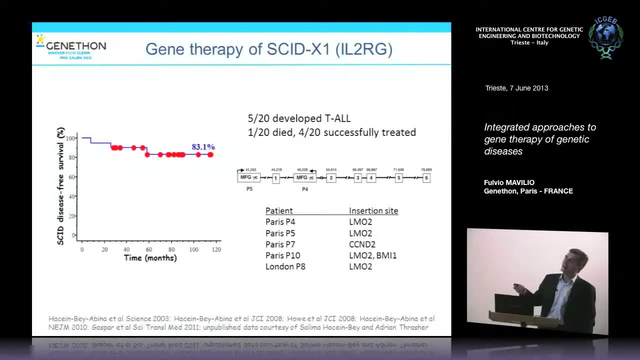 Of course the vectors are not perfect, Of course we don't want to cause insertion or oncogenesis. And well, this is the same thing. This is the survival after 10 years of these patients And these are the insertions into one oncogene. essentially, 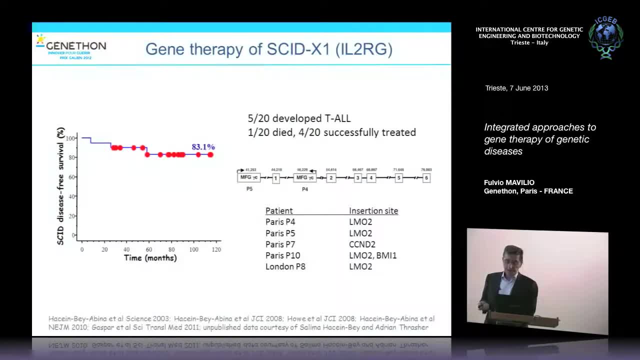 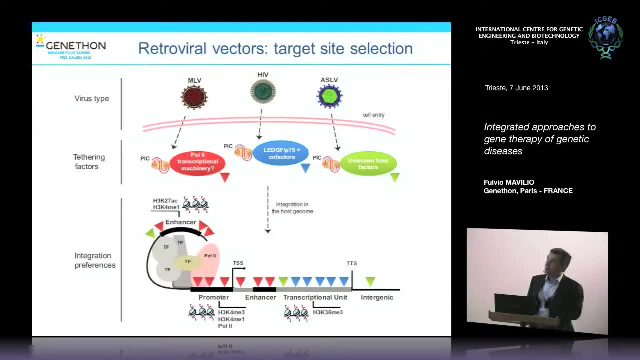 that caused the leukemias in four patients in Paris and one in London. Something causes leukemia in Paris more often than London, and we don't understand why. So what we know, of course, these days is that, of course, we don't know exactly what's going to happen. 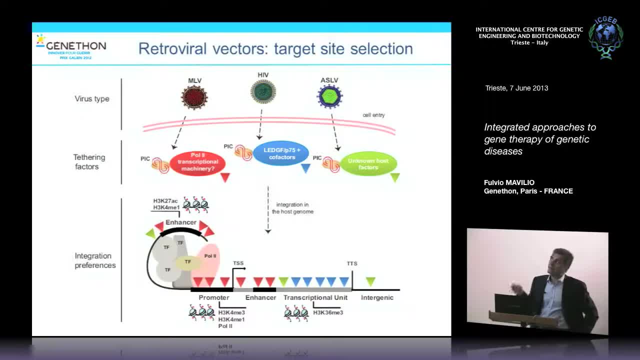 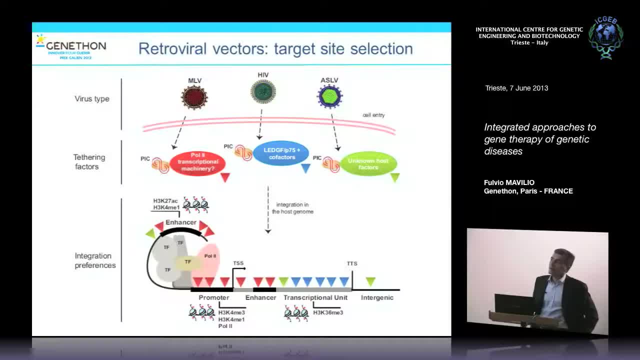 More. only leukemia viruses tend to go into regulatory elements of gene. They hit regulatory elements, They hijack essentially regulation of genes by using their own regulatory elements And this, of course, is a type of vector that is very much prone to cause upregulation of genes. 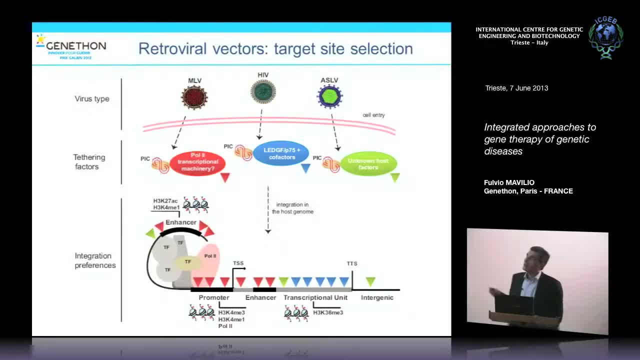 And if these genes are proto-oncogenes, this might have a consequence. Lentiviral vectors, on the other hand, have completely different characteristics. They tend to go into, not in promoters and regulatory elements, but here in blue, into the transcribed portion of genes. 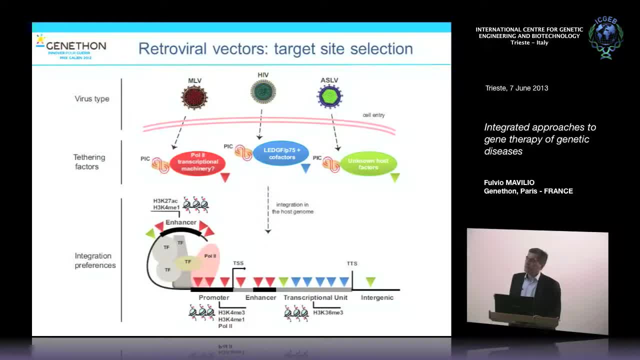 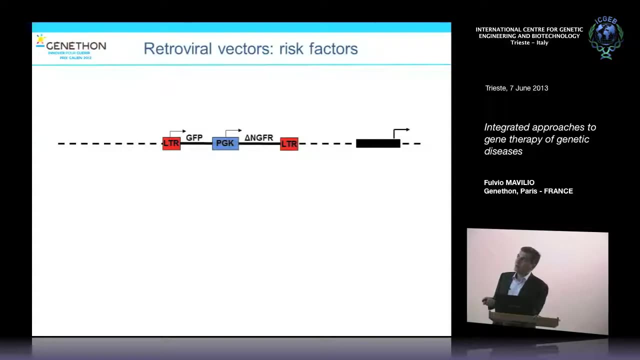 so essentially into exons, away from regulatory elements. So simply looking at the integration characteristics, you can predict that this would be much safer vectors, And so far they are in the clinical applications that we know. So, while in the case of more leukemia, virus-derived vectors, 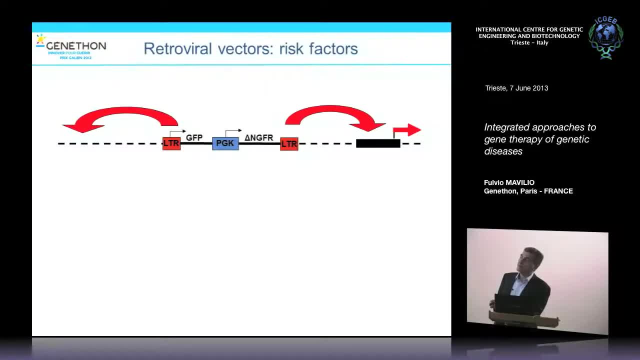 the problem and the risk factor is due by, as I said, upregulation of genes. So it is a dominant molecular event In the case of lentiviral vectors, self-inactivated with cellular promoters away from regulatory elements, probably the frequency. 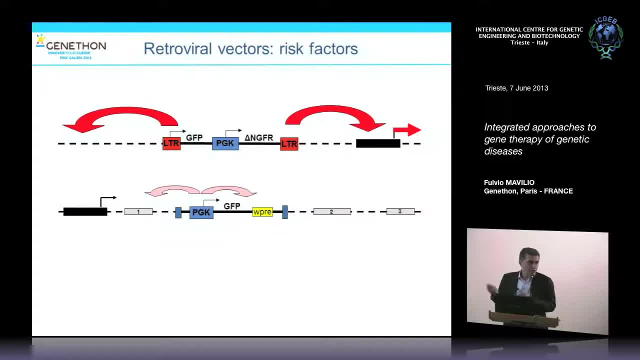 of having this type of event is much, much lower. All this was proven, of course, in vitro and animal models. I'm not just predicting things here. There are other problems for this vector, which is called. they are prone to induce alternative splicing. 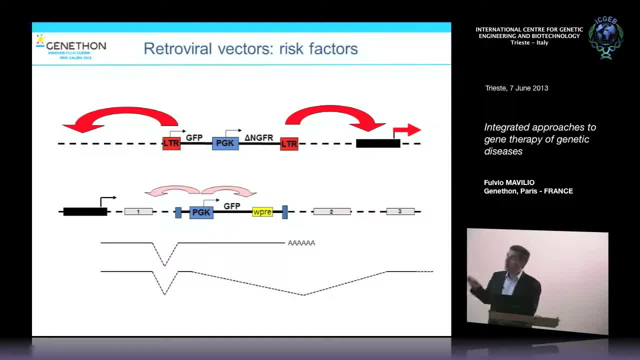 and premature termination, which is one of the problems that need to be addressed, But altogether all the preclinical models that we have show that lentiviral vectors are much safer into human hematopoietic stem cells or mouse hematopoietic stem cells. 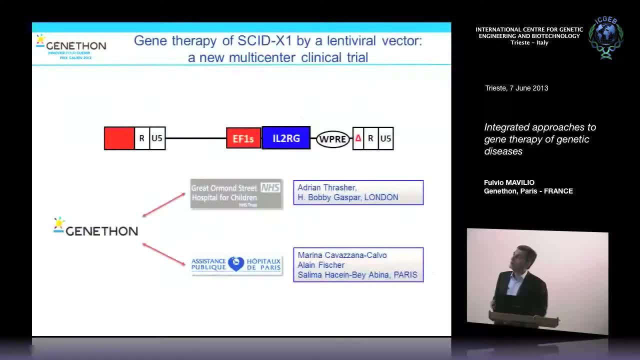 or monkey hematopoietic stem cells. So what we're doing now at Genedon is to rebuild the vector for the exoskeleton. We're going to take it, the IL-2 common gamma receptor, into the framework of self-inactivating lentiviral. 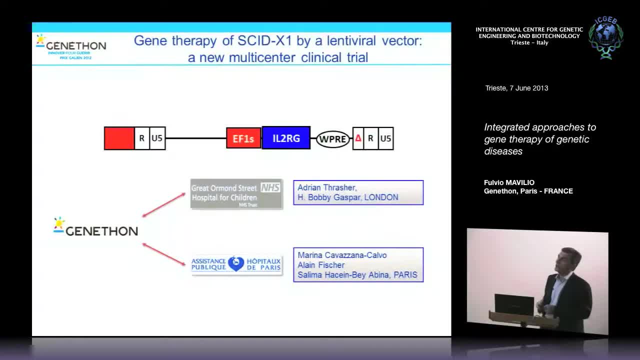 vectors with elongation factor 1 alpha promoter that has excellent genotoxic characteristics. And this will be another clinical trial which will be carried out again in London and Paris by the same clinical groups, And we hope to be ready to do this starting in 2015.. 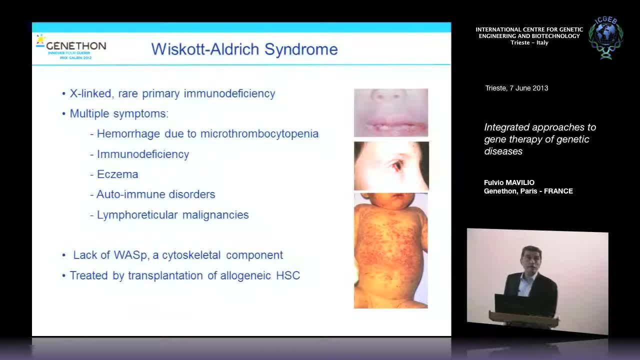 The last two things, I would probably show only one, because we are really running out of time. The last thing that I will show you is something that is already in the clinic, And it's an application of a lentiviral vector, And it's for this type of disease. 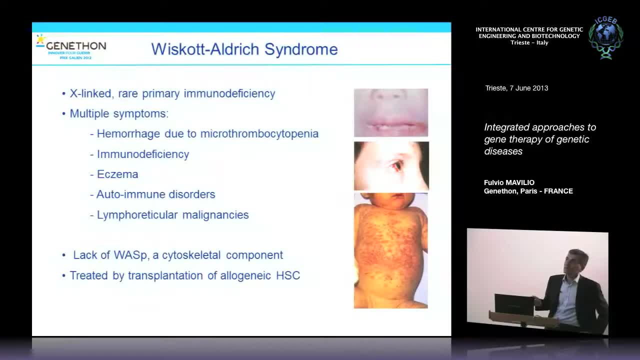 It's called Wieskot-Aldrich syndrome. This is another immunodeficiency, X-linked. It has multiple symptoms. It is due to lack of this protein- It's called Wieskot-Aldrich syndrome- protein, which is a cytoskeletal component which 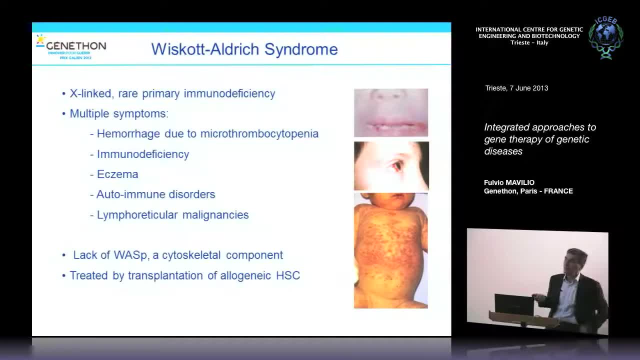 is particularly important And for supporting the so-called immunologic synapse. So lack of this protein is deleterious for T cells, for B cells, for a number of other cells, including platelets, And so the result is an immune deficiency. 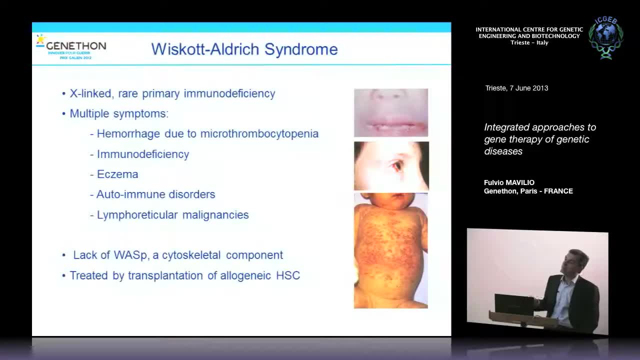 with a lot of other problems. It's normally treated by transplantation of allogeneic stem cells from fully compatible donors when you have them, And normally this is less than 1 third of the patients. For the others, there is no cure. 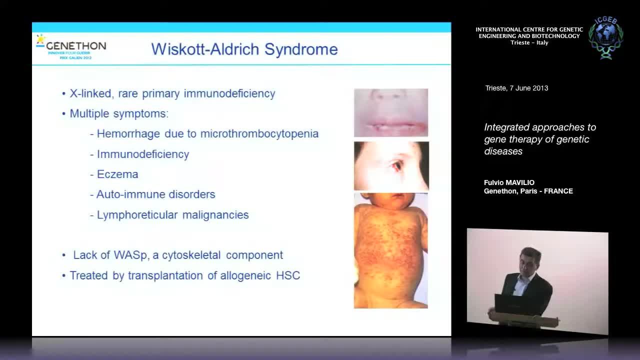 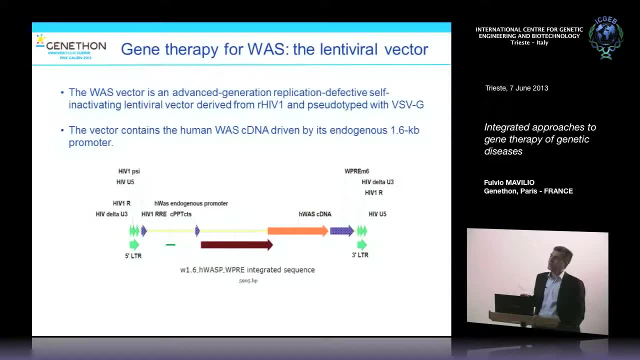 These are the symptoms. The eczema is really a hallmark of this disease. What has been developed? This was done. I followed the development of this from both sides of the Alps, So this was started when I was in Milano as a collaboration between the two teledons. 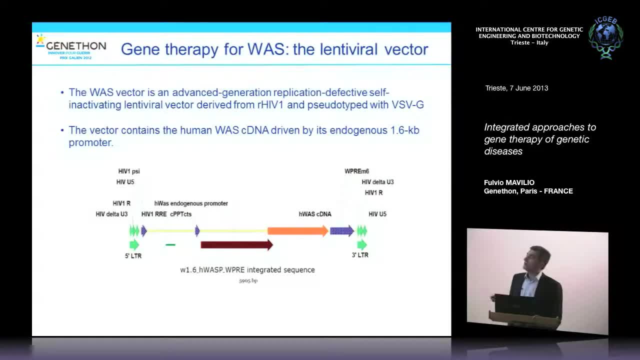 So TGET and Genadon, And now I'm there On the other side, On the other side, to finish this, But it's essentially an antiviral vector with the WASP cDNA and the WASP promoter. This is a design that, as I said, 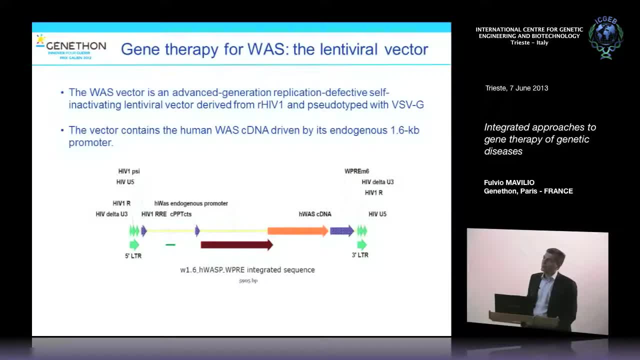 was developed by the two groups together and essentially with the help of Adrian Thrasher. So this is a rather big gene, rather big cassette. This was developed as a full antiviral vectors. All kinds of preclinical studies It was done. 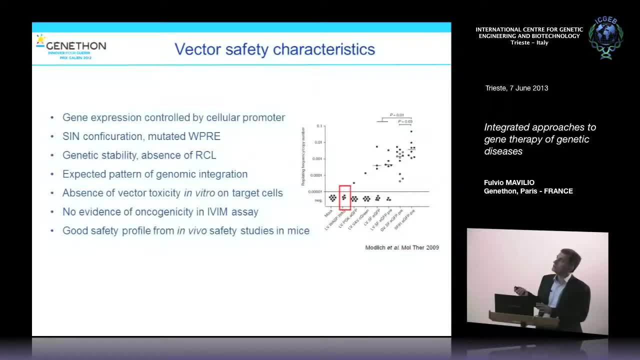 And I don't have the time to tell you this, So I will just go very fast. But in a very good- let's say validated in vitro- assay of genotoxicity, this vector scores exactly like non-transduced cells. as opposed to other vectors that score, 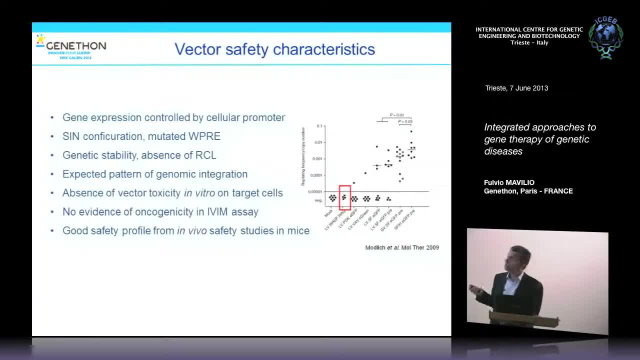 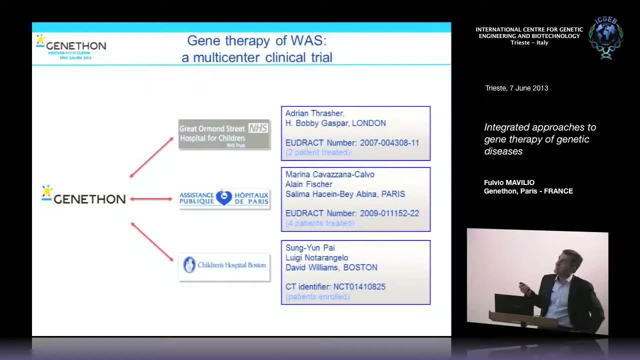 positive in this in vitro induction of a chronogenic expansion, which was developed by Chris Baum a few years ago And it's now It's done. It's standard. The same happens in vivo And now this is a clinical trial. It started already in London. Two patients have been treated already in Paris. Four patients have been treated at the Children's Hospital in Boston. Patients have been enrolled but not treated yet, And everything is sponsored and coordinated by Genetone And the vector is produced in Paris and sent to all the centers. 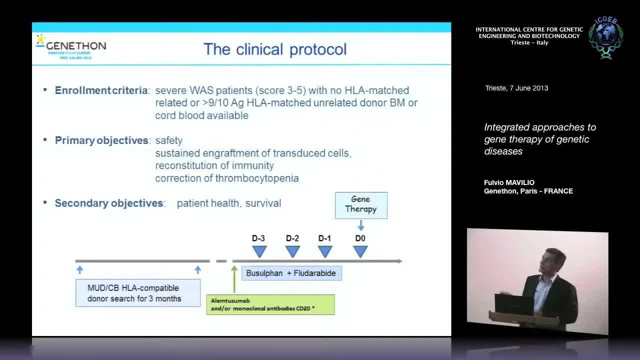 I don't know how many of you are interested. I'm interested in this type of details, But of course patients are treated before infusion of genetically modified cells with, rather, I would say, conventional chemotherapy. This is the trial. The enrollment criteria are severe patients. 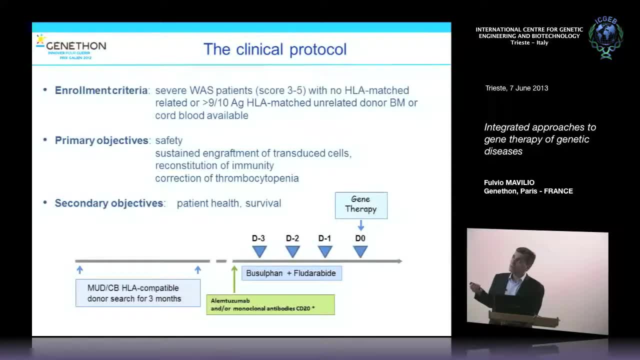 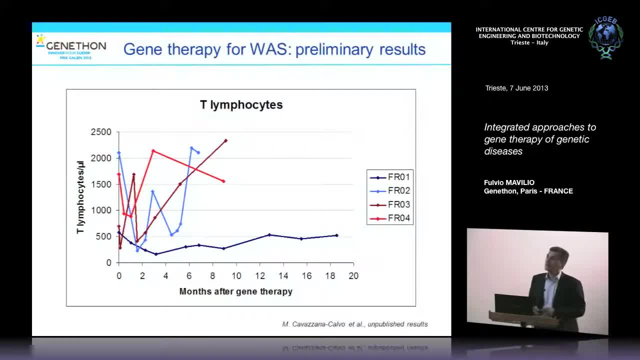 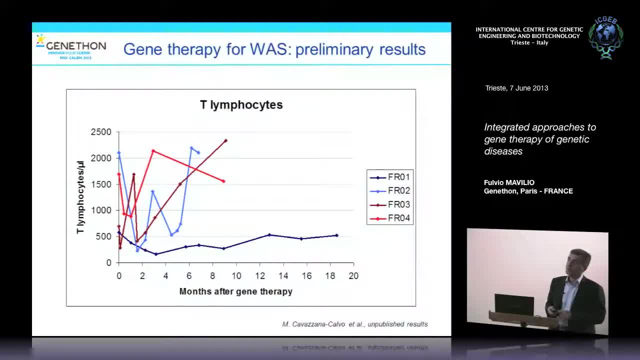 So this is the clinical results of the first patients. I must say that the same trial is carried out. I mean the same trial. a very similar trial with the same vector is carried out at the same time at TGET by Alessandro Iuti. 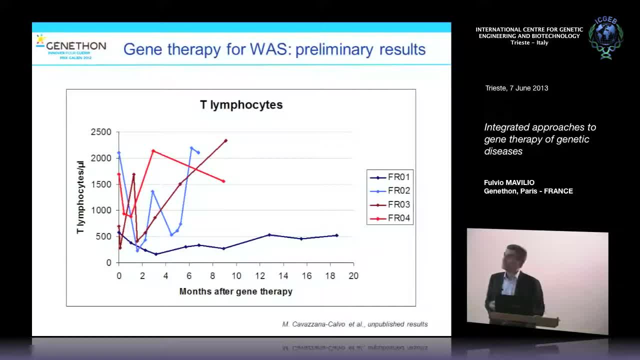 He also treated six patients. Results are very much comparable. So this is very reassuring, very safe in all cases and clinical efficacy is already obviously there. So this is the recovery of T lymphocytes in the four French patients, which looks very good. 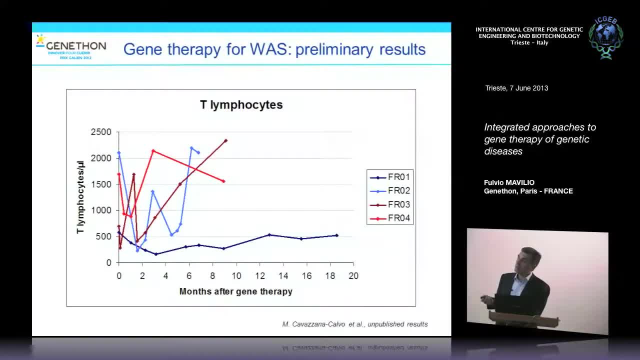 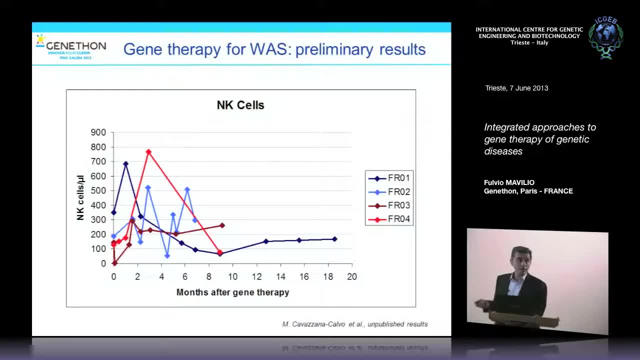 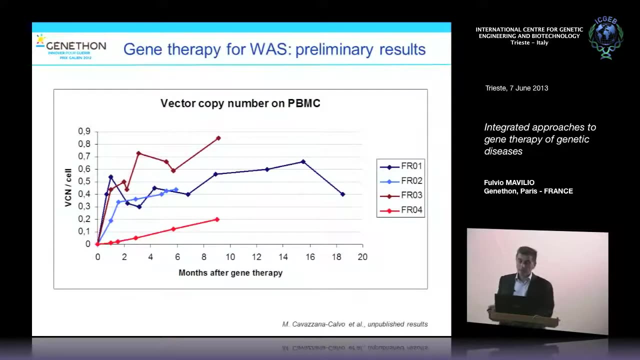 We go from very low level of T cells. These are B lymphocytes, These are NK cells. So you have recovery of everything, including NK cells, and you have recovery of platelets. I don't think I have. No, I don't have the slides. Platelet recovery is much slower, but it's essentially there Between eight months and 12 months after transplantation. And vector copy number. this is important, So this type of therapeutic efficacy is obtained if you count how many copies per cells are in peripheral blood of these patients. 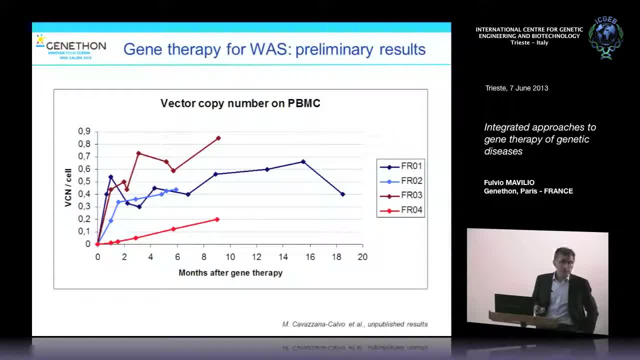 at the vector copy number. that is very reassuring. Essentially, the crude vector copy number is lower than one. Transduction level is between 30 and 40%, which means that the number of cells that we said. on average, these cells contain between one and three copies of the vector. 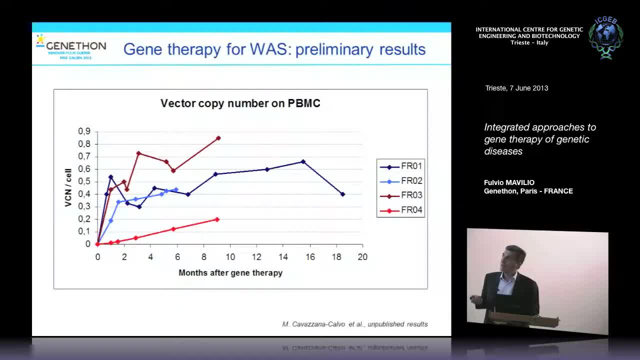 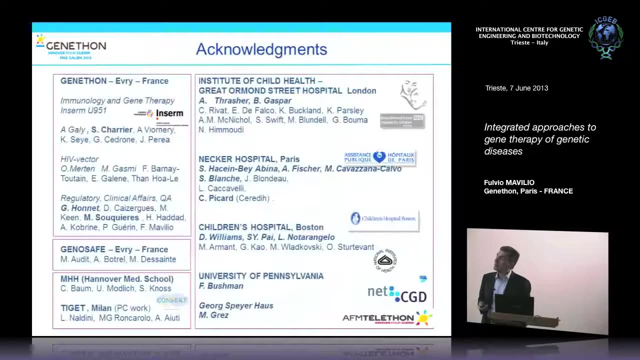 So this is what is the therapeutic level, apparently, for this type of vector, this type of disease. I will skip the last trial because I'm sure that you're already pretty much dead, So just let me go to the acknowledgements for the second part. 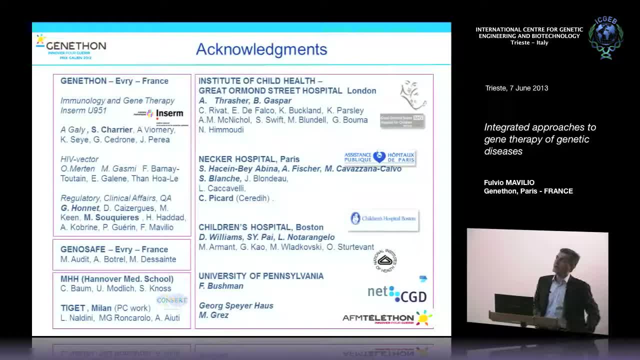 And, as I said, all this is done again by an enormous number of people. This includes many people in Genedon and particularly Angali. I have to say she's the project leader and she was really instrumental in developing this whole machine and particularly the production process. 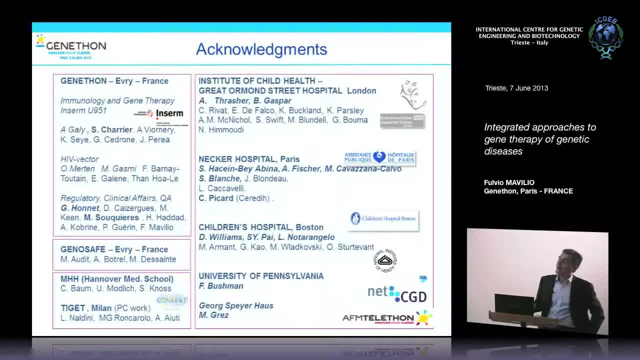 which is working beautifully, And people in Hannover that helped us for the preclinical studies. As I said, this was developed together with TIGET, in particular with Alessandro Iuti and the clinicians that are doing this, which are in Paris, in London, at Children's Hospital. 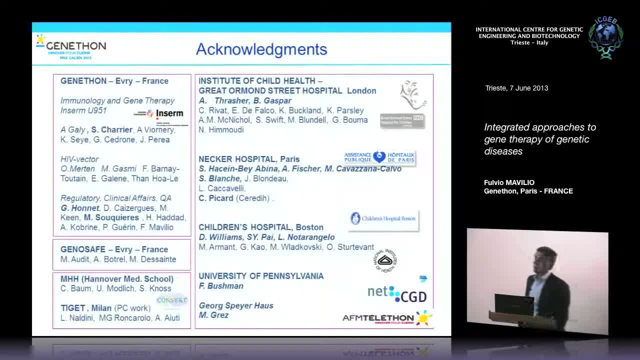 Let me also mention Rick Bushman, who is helping us in analyzing, with very fancy type of technology, the dynamics of the engrafted stem cells into these patients. I think I will stop here If you have any question. thank you very much for your attention.